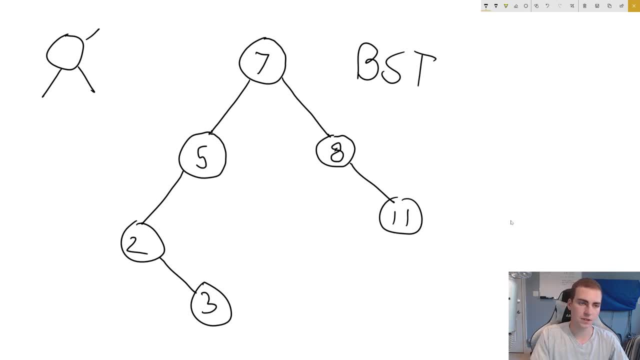 parent node has at most two children. So if you say this is the parent, which we'll say is p, then I guess I'll actually I'll just write them right on here: These are the children, right? And that it has at most two. it can have none, it can have one, but it can have. 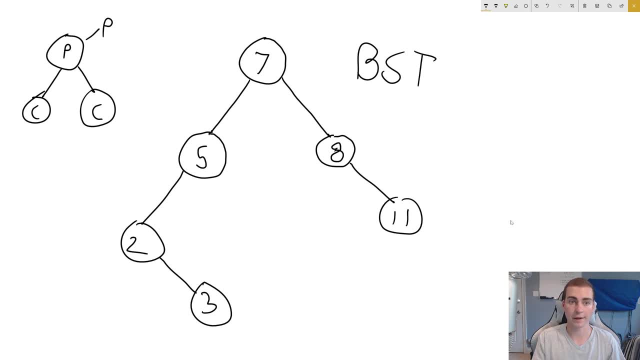 at most two, And that's all a binary- or I guess a binary tree is. it just has two children for each parent. So now, if we call this one the parents, it can have at most two children, And you can keep going in. each node has at most two children. that's all a binary tree. 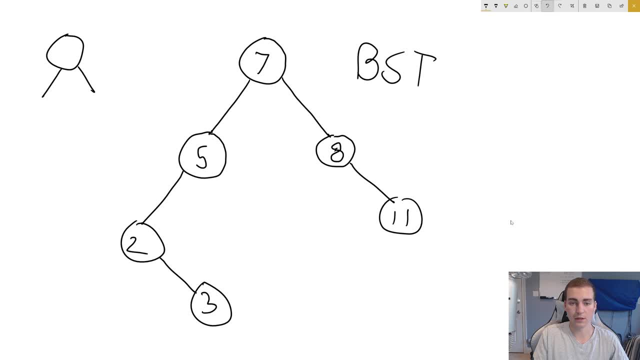 is. So you can see this big tree that I've written in the middle of my screen is a binary tree, And that's because at most we have two children to each parent, node. So if you say this is the parent, You can see we have child one and we have child two and then the rest of them only. 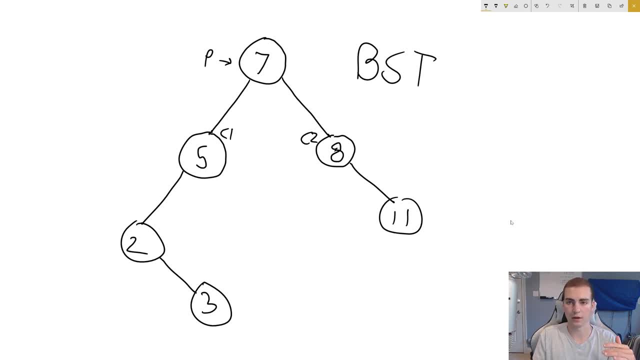 have one child. Now, a child is just the node that kind of proceeds or comes after or is connected to one of these parent nodes, And that's kind of some terminology I'm going to be using here now. Now this is called the root node. Now, the reason it's called the: 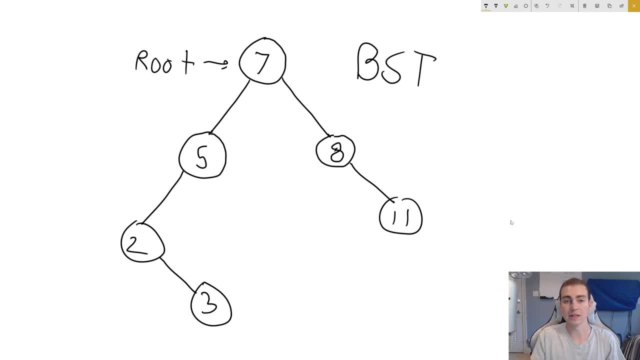 root is because it is the start of our tree. it has nothing that comes before it And it's actually the only node in our tree that has no parent. So we call it the root. That's important, because I'm probably going to use that terminology a few times. So anyways, 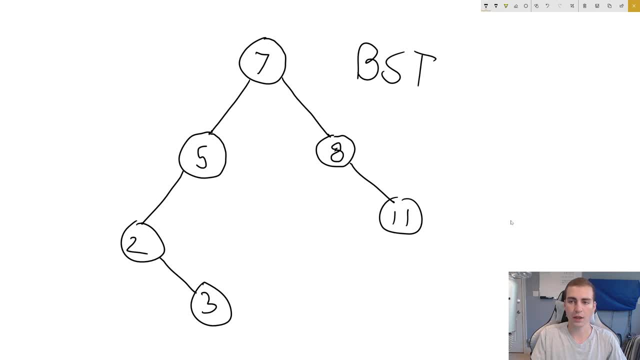 that is the root node. I'll just erase that for now. Okay, so now that we know what a binary tree is, what is a binary search tree, also known as BST? Well, a binary search tree now satisfies another property. Not only is it a binary tree, but it also is a search. 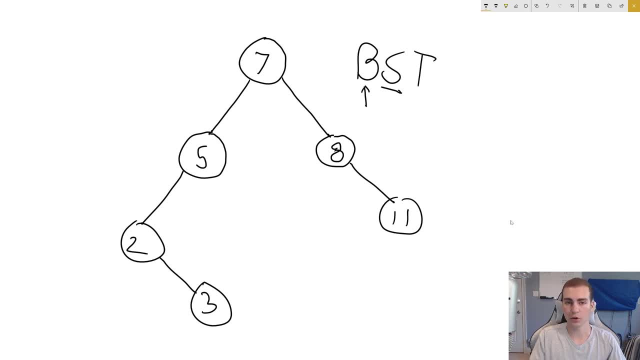 tree, which means that we can find elements in it very quickly. Now, the way we do this is because every child that's connected to this tree in a specific way. So looking at our root node here, we can see that the left child 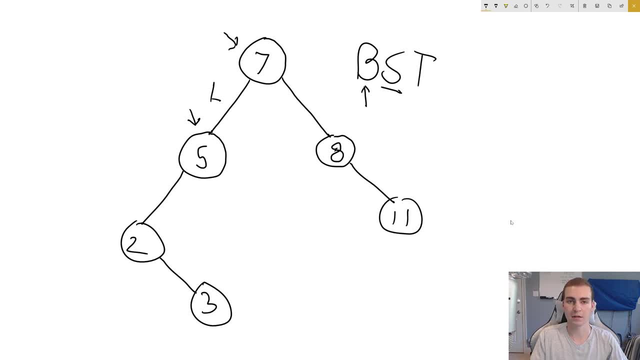 which would be this one here. so five is always less than the root node. So you can see, five is obviously less than seven, and eight, which is our right node, is always greater than the root node. So the way this works is when we add in new elements based on where we're. 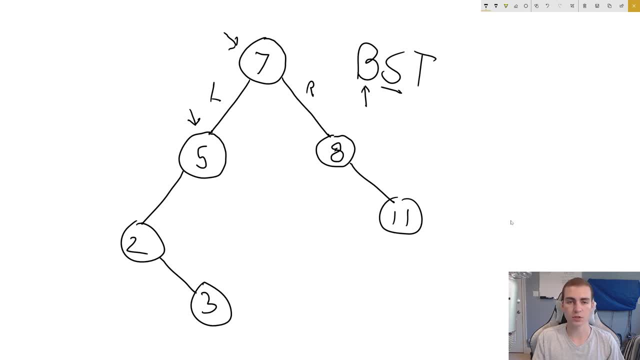 adding them in the tree. they're always going to put themselves in some kind of order, So that's very quick and easy to find certain elements in the tree. So if you look at five here, you can see that two- since it's less than five- goes to the left of it, And three. 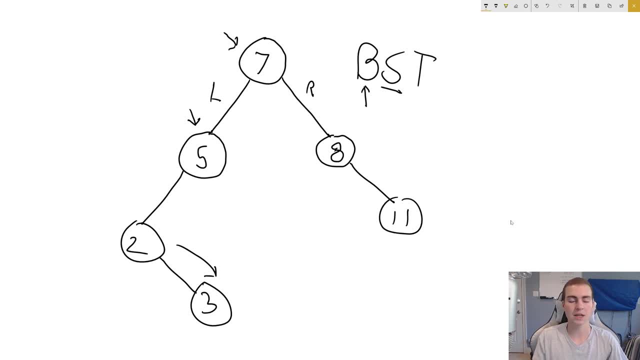 over here. since it's greater than two, it goes to the right of it And that is kind of the way that we add elements in and the order that we maintain in this tree. So having that property satisfied, where every left child is less than the parents and every right. 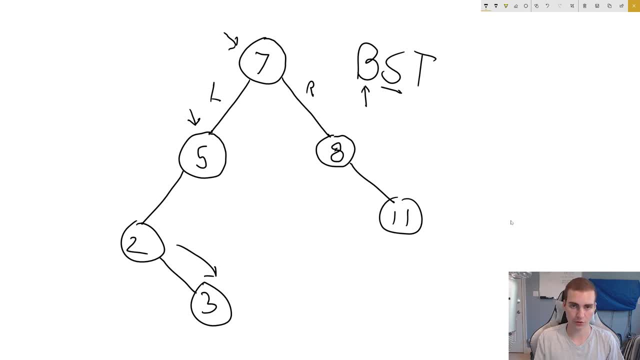 child is greater than the parent is what makes this a search tree. So those two properties combined gives us the binary search tree. Alright, so let's start discussing binary search tree properties and how we can actually create one of these trees. So I'm just gonna. 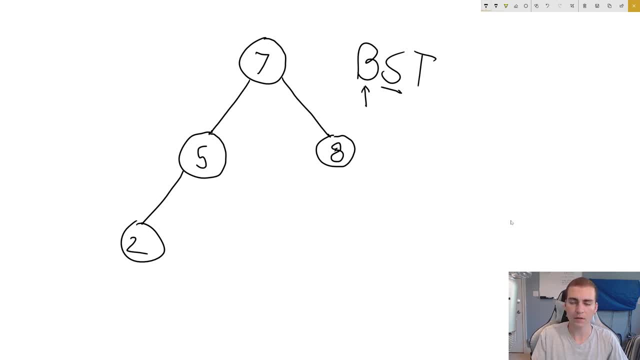 erase a few nodes here so that I can add in some more ones. Let's say, we have a tree that starts off looking like this: So we have that root node is seven, then we have five, then we have eight, then we have two. Well, how do we add elements into this tree? Well, what? 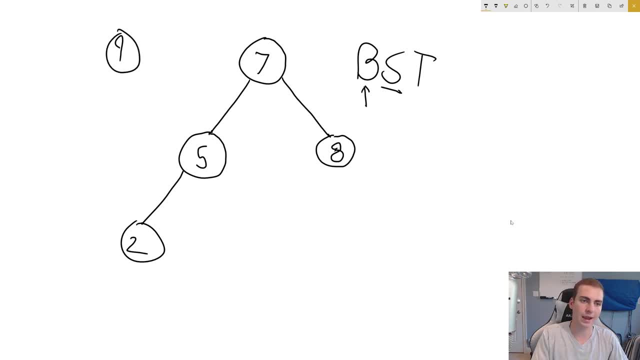 we do is, let's say, we have the element nine and we want to add it into this binary search tree. Well, when we add it, we need to make sure that the same binary search tree properties are satisfied. So what we do is we compare it first of all to the root node and we say: Okay, is this? 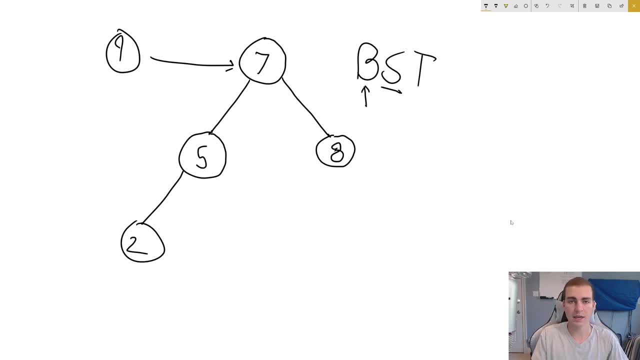 value greater than or less than the root node. In this case it's greater than, so we move to the right. Now, if there was no root here- or sorry, not root- if there's no node here, we would just add nine in, So we could replace, like where eight is with nine, if eight wasn't. 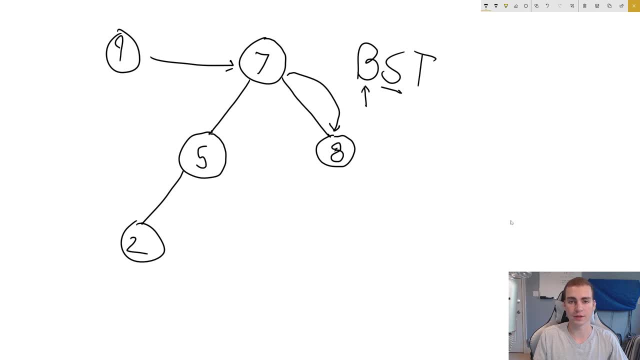 there, But since there is one here, we need to figure out where we're putting this based on this node. So we look at eight and we say: is nine greater than or less than eight? Now, since it's greater than what we do is, we move to the right again. we see that there's. 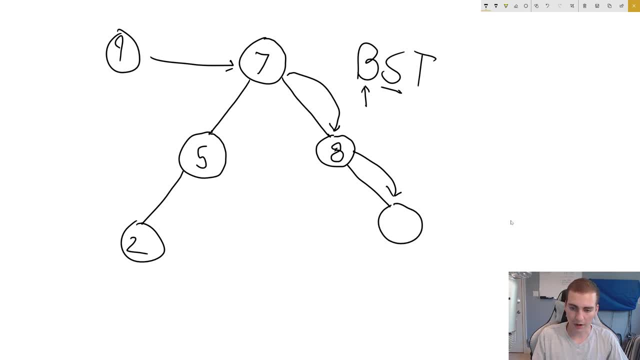 no node here. So there's room for us to place nine, And we put nine right here as the right child to eight, And that's how we add elements into our binary search tree. Now let's do another example with the element three. Now you already know where three goes, because 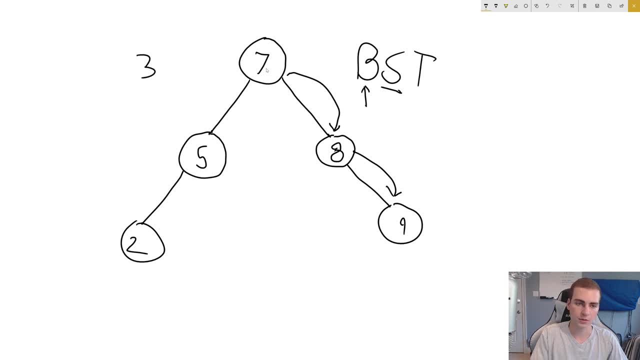 you saw me show it, But let's do kind of the process of how we add it. So let's say we want to add three into this tree, we do the same thing. we compare it to seven. we say is less than or greater than, it's less than. 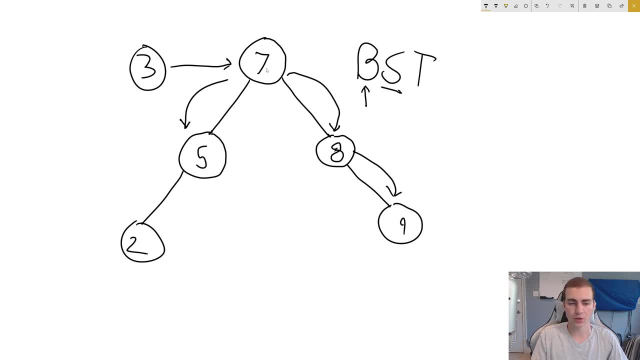 So we go to the left. is there room for three? yet No, there's not. So we compare it to five. we say: is it less than or greater than five? Well, it's greater than five. So we go to the right. Turns out there's no other node there, So we can go ahead and add three And 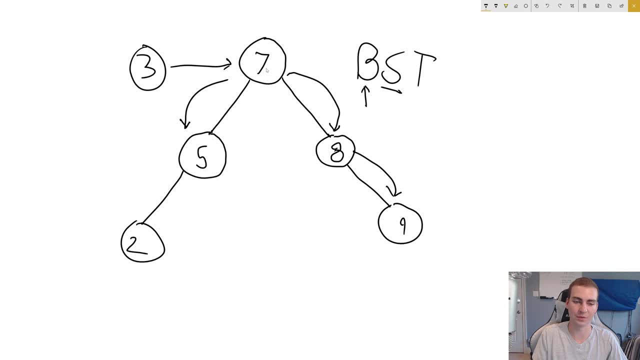 now are. sorry, what am I saying? What do we put going to the right? Sorry, we go down to two. we go to the left because it's less than five- Yes, I'm thinking correctly. And then we say, okay, is it less than two or greater than two is greater than two, So we add it. 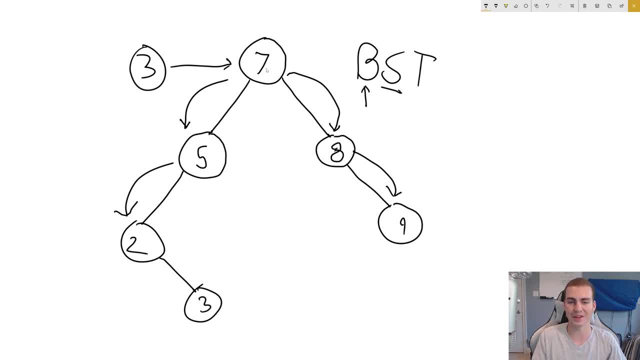 as the right child to two, to my apologies on that one there, guys. So that is how that works And that's how we add elements into the binary search tree. Now, this is pretty straightforward, So let's just start by constructing one from scratch, to make sure that everyone understands how. 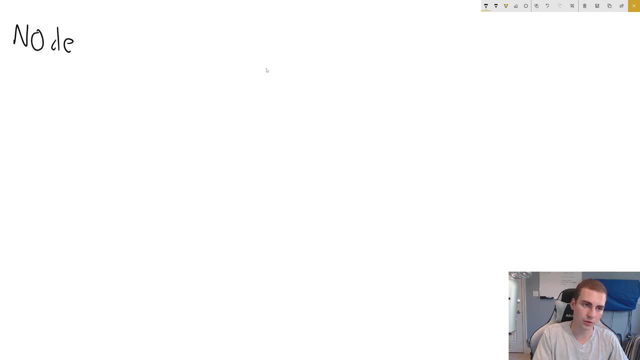 this works. So our nodes- just going to do a quick note here- have a value. they have a left node, so a node that's attached on the left, and they have a right node. Now, when we start off our tree, we don't have any nodes. So what we do is, let's say we want. 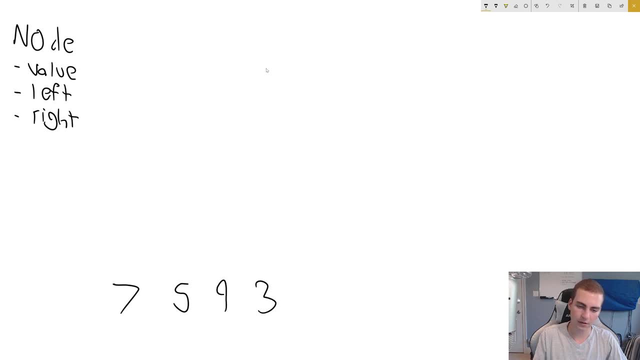 to add the numbers seven, five, nine, three, two. these are the numbers that we want to add into our binary search tree. How do we do this? Well, we start with seven, And since there's currently no nodes in our tree, seven immediately just becomes our root node. So we write seven here. 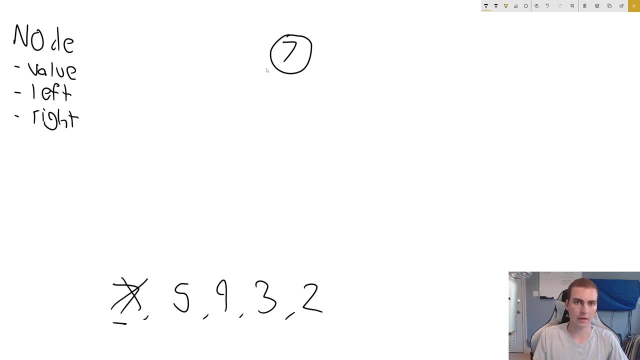 And we throw that one like that: Now, seven is gone, we've added that one into the tree. Now we move on to five, And now we repeat the process I've just talked about. So we say, Okay, let's compare it to seven. is it less than or greater than seven? is it less? 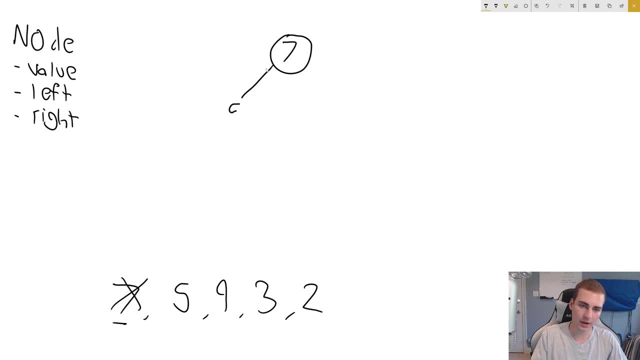 than or greater than seven. it's less than, so we're going to add it right here to the left of seven, And this is what's going to be now the left node of the value seven, or on the node seven. this is the left shot. Alright, so that's how we do that. Now let's 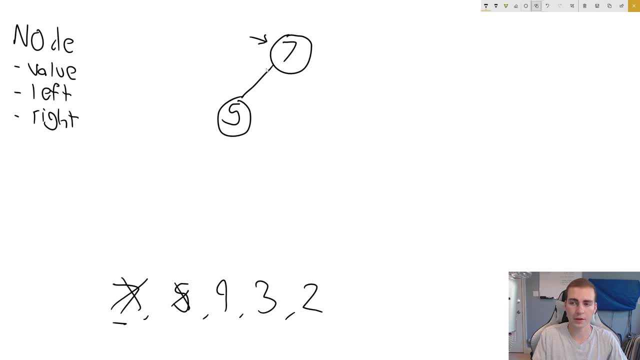 add nine. Okay, so we compare it to seven. we say: is it greater than or less than? well, it's greater than, so we go ahead and add it to the right side here, And now we have nine. Okay, nine is gone. Now it's time for three. Alright, so let's add this in now. 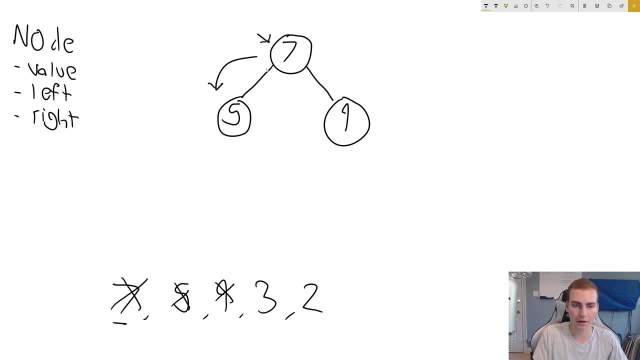 So we look at seven, we go to the left because it's less than. we look at five, go to the left because it's less than, and we add three, like that, And now let's keep going And let's add two. So when we do two, we do the same process. here we go left, left. oh, it needs. 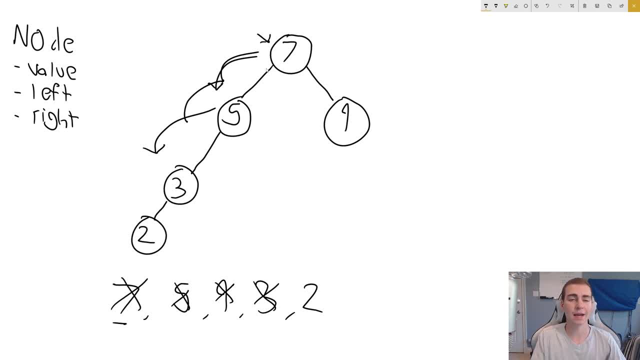 to go left again And then we add two right there. Now let's add in one more number, just to show kind of how this works. So let's say we want to add six now, Well, let's, I'm just going to erase some of these lines. 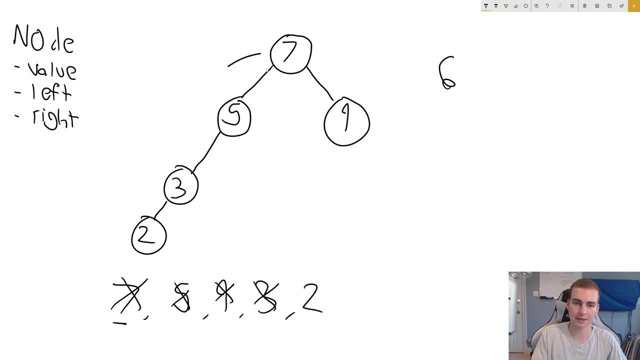 Let's do the same process again, Then compare it to seven. is it greater than or less than? it's less than so we go the left. compared to five: visit less than or greater than it's greater than So we go to the right. 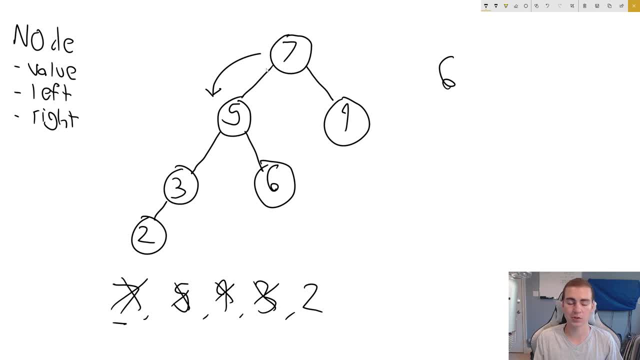 and we add six, And that is how we construct this binary search tree from scratch. The first element just immediately becomes that route, And then from there we just compare it to each node. we USA, do we go to the left, Or do we go to the right? and we keep going. 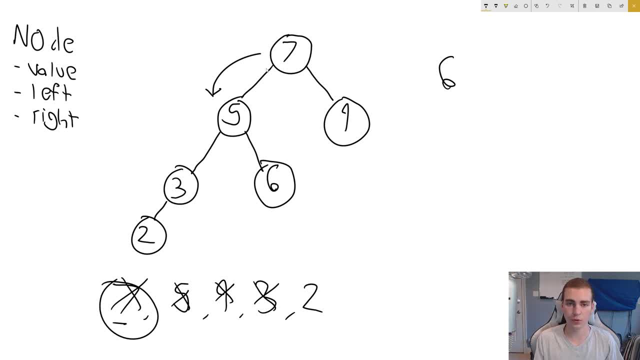 through there until eventually we have room to add in our note. Now, this is just basically how it works. So let's talk about kind of more of an implementation of this now in code, because this has all been kind of abstract. So let's just erase some of this stuff down. 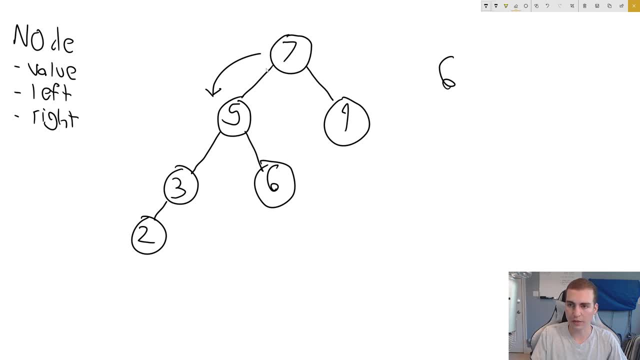 here. So the reason I wrote this node thing here on the left side of my screen is so that we know what each of our nodes have. So what we're going to do is, in our program we're going to set up an object. it's going to be called node. what we're going to do is each. 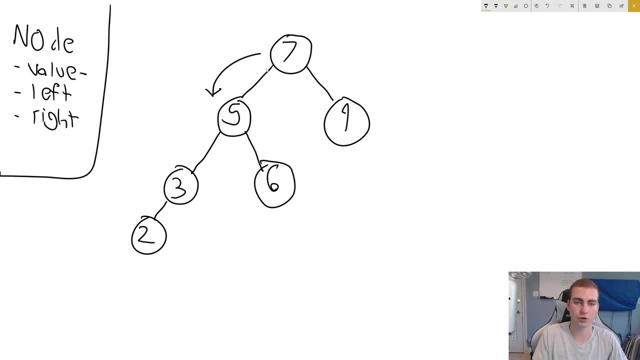 node in our binary search tree is going to have a value which could be, you know, 759,, whatever it is, And it's going to have a pointer to a left node and a right node. So essentially what happens here is we actually store this node in, you know, the left property of seven. 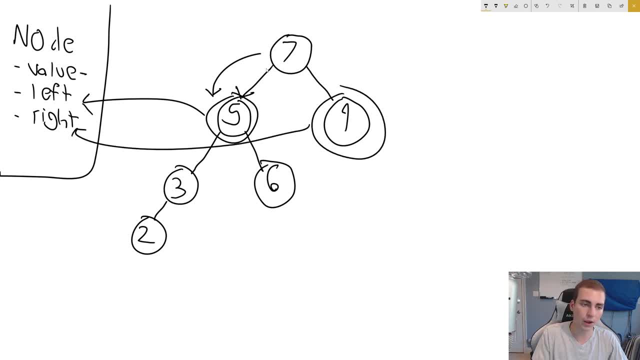 and we actually stored this node, which is nine, in the right property of seven. So when we actually want to loop through and look through our binary search tree, we can do this recursively, Alright. so what I'm actually going to do now is program an implementation. for a binary search tree. I'm just going to do this in Python before I use a class tag, And of course I think it's going to be much easier if you have a class tag. let's say, for my class. So let's start with the class tag. So I'm going to set up a class tag here. 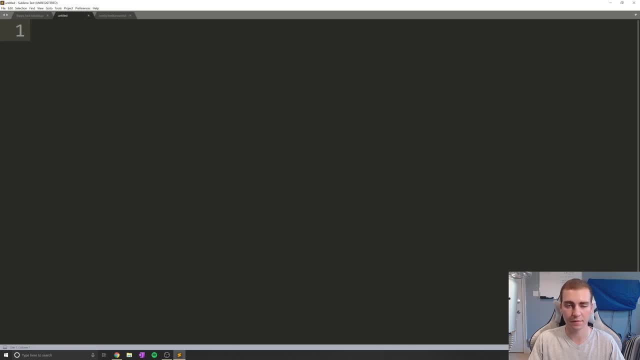 to write these out, But I was finding that it's getting kind of messy And my handwriting obviously is not neat enough to do like long bits of code, which is kind of what we need to do here. So I'm just going to do some kind of pseudocode Python like programming of. 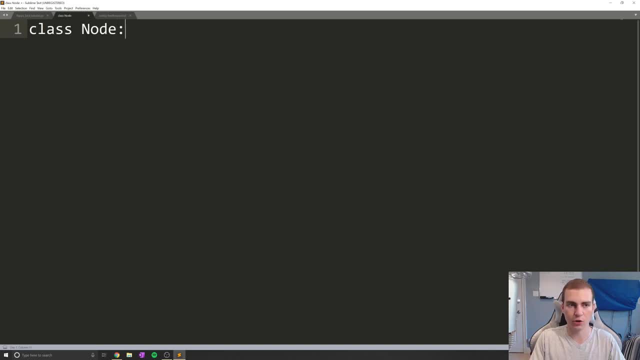 a binary search tree. So the first thing that we need to do is create a node class. So I'm going to say there's a class node, it's going to have a few properties. we're going to say: define, underscore, underscore, knit, underscore, underscore, And what we're going to do in. 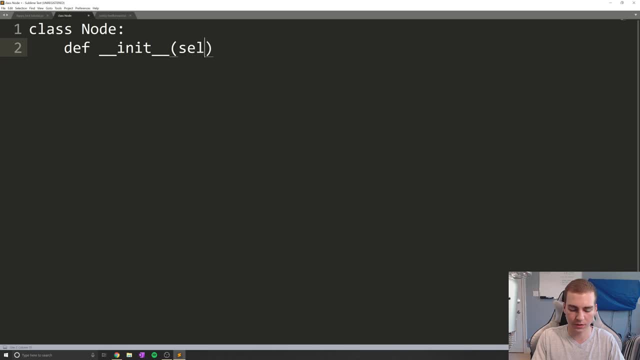 here is simply define a value for this node. So let's say self, we'll say value, And then what we're going to do is add some attributes. So we'll say self dot value equals value, self dot left equals none, And self dot right equals none like that. Now let me just save. 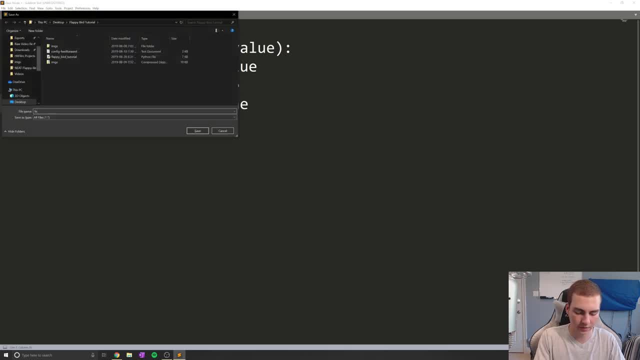 this as a Python file, So it's called test up pi, because we're probably not actually going to run this. save it like that. So, anyways, that's what we have. we have this, no class, And this is really all we need. 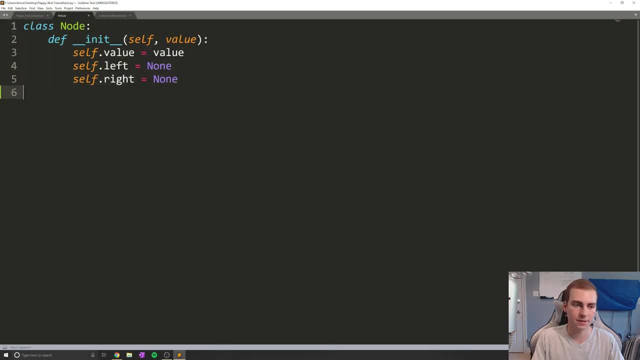 For our node class. we have a value and we have a left and a right. Now the next class we're going to write is going to be called BST, or binary search tree. Now, what binary search tree is going to have is just simply one property, So we'll go into a net underscore. 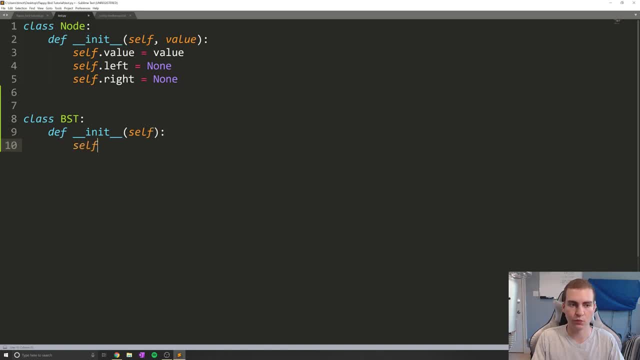 underscore. And then in here, what we're going to do is simply just define a root. we're going to say self dot root equals none. Now, what this is going to mean is essentially, when we first create a new binary search tree, there's nothing in it, And this root node 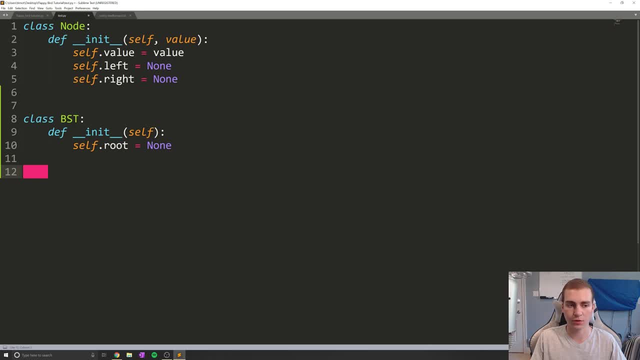 is the only thing that we actually want to keep track of in our binary search tree. it's gonna start off at none, But what the root node is is that first node in this, the tree. So when we actually start adding elements into the tree, what we're going to do is the first. 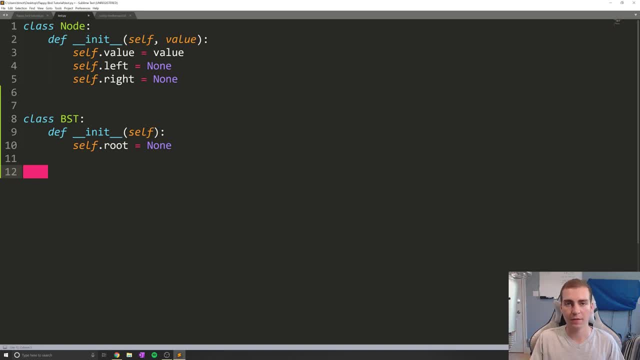 element we add will become that root node And then from there that root node will have a left and a right And then all those other nodes will have lefts and rights And we can access those nodes by going to the left of the root node and the right of the root node. 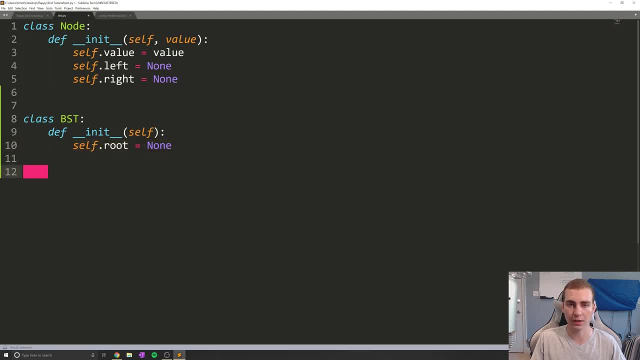 and so on. So that's why we only need to hold a root node here in BST. So we're going to add a new node to our binary tree. Now, the first method that I want to program here is going to be an add method, And the add method is going to well add a new value into our 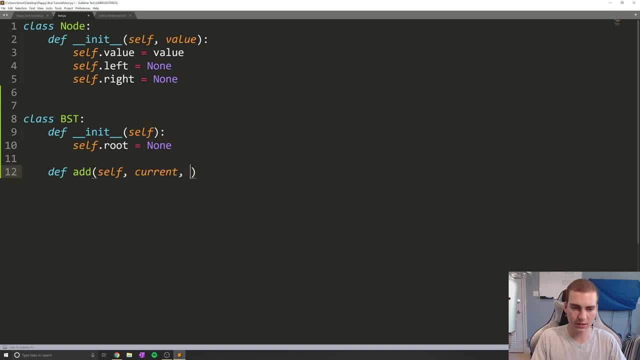 binary tree. Now, what we're going to take in here is current, And we're also going to take value for what value we're adding to our search. So what I'm going to do in here is just kind of start programming this And then, hopefully, I'll walk you through this. 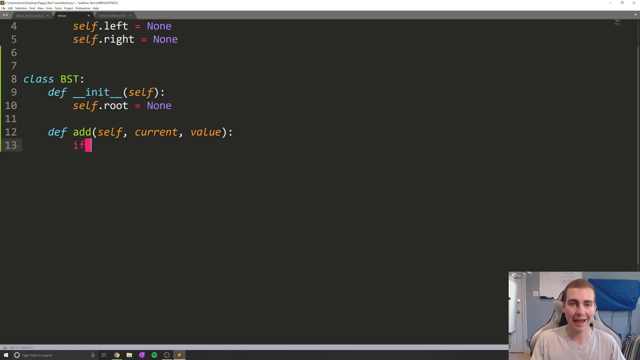 as we get go through it. The first thing we need to check when we add a new node into our tree is if we have a root node or not. So what I'm going to do is I'm gonna say if root. actually I'll say if not root, which means you know, like if root is equal to none. 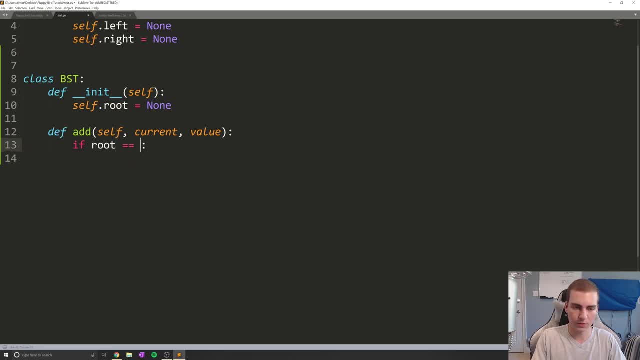 so I guess I can simplify that and just say: if root equals equals none, then what we're going to do is just simply make whatever this value is a new node. that is going to be the root. So we're going to say self dot root, which I guess this needs to be. self is going. 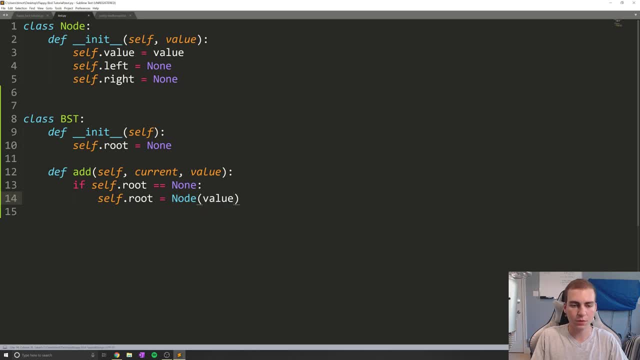 to be a new node, And in here we're just going to put value. So what this is going to do is construct a new node, as we can see here, and we're going to store that as the root node, because we don't have one yet. that's what we need to do Now. otherwise, 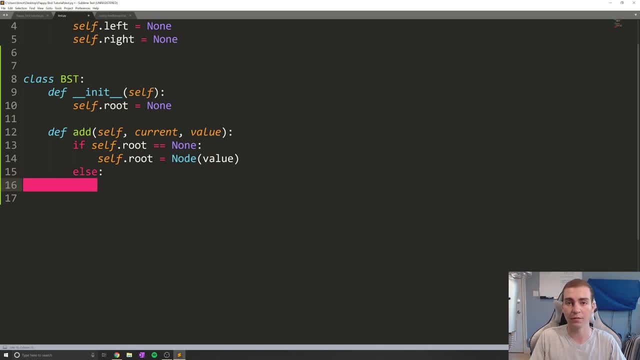 what we're going to do is actually write kind of recursive method of finding out where this node needs to go, because it needs to be in the correct sorted order, needs to be there to the left of the root node or to the right of the root node, And then, after all those, 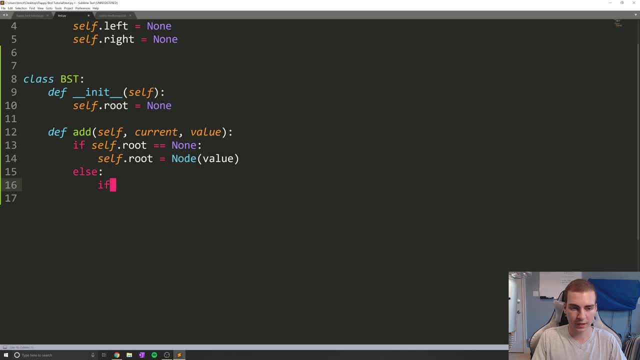 children and everything it needs to be in the correct order. So we're going to start with the root node And then we're going to say if value is less than, in this case, current dot value. Now I should say here that what current is is going to keep track. 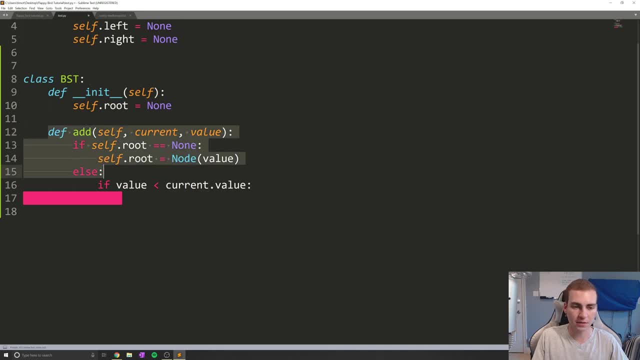 of the current node that we're looking at, because I'm actually going to make this method recursive. you're going to see how that works in a second, But current is going to start off as the root node for our binary search tree, So we're going to start as that route. 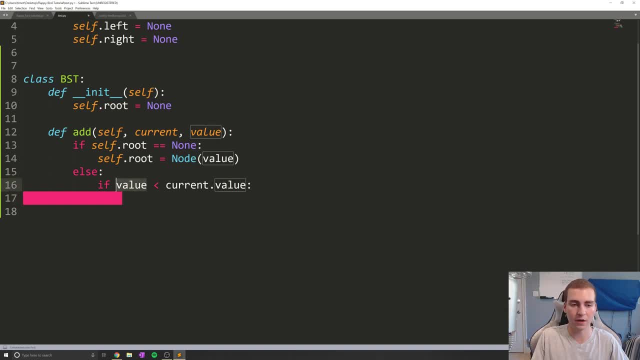 So maybe we say that value seven, we're going to compare the value that we're trying to add to that root node to start, and then do something with it, Based on if it's less than or greater than. So if the value is less than what I'm going. 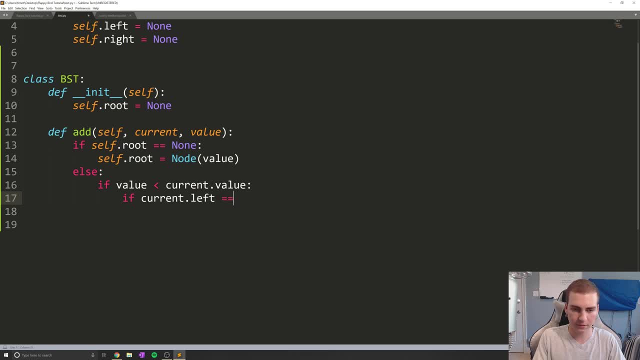 to check is if current dot left equals, equals none. Now, if it does equal none, that means- and I'll do a quick illustration here so that we can see kind of how this works- So we have this root node. let's say, maybe this is seven. I'm just drawing with my mouse, So give me. 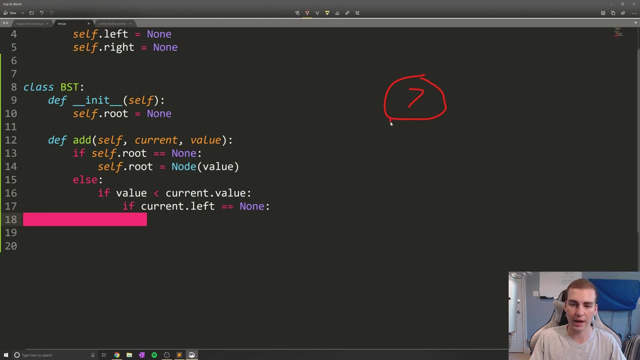 a break here. we compare it to seven, you know, and we go. now we want to add our node. we check if the left of seven, if it's no or not, or if it's none. if it is, what we're going to do is just add the node in there. 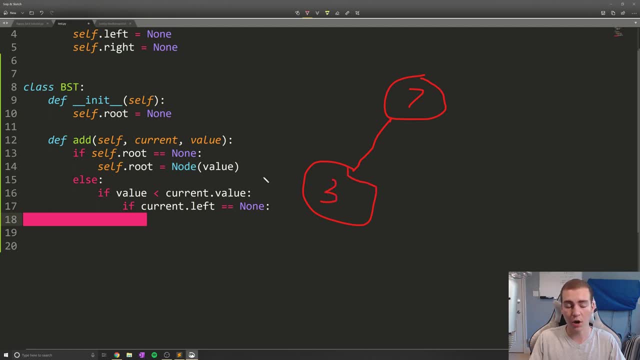 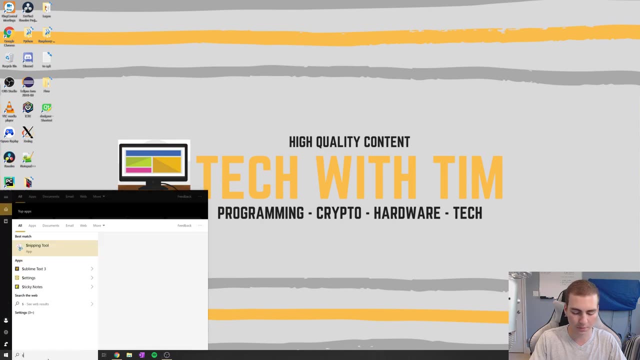 So let's say we wanted to add three. well, we'll just put it there. Now, if it's not none and there is a node here, then we need to do something else. So, anyways, let's get out of this. I did not mean to do that. Okay, so if current dot left equals equals none. 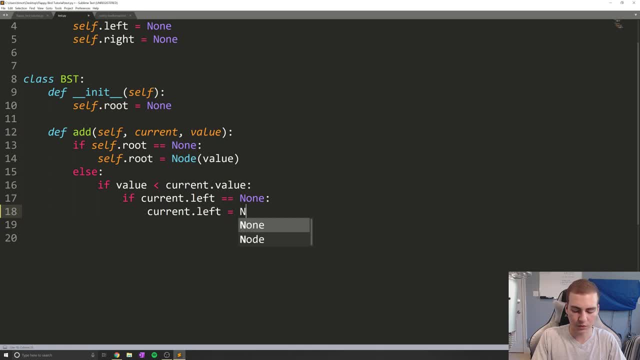 then we're gonna say: current dot left equals node value, And that's as easy as that is to add the node on the left side of the tree. Now, if it's not none, what we're going to do is we're going to say else: self dot, add current dot left. 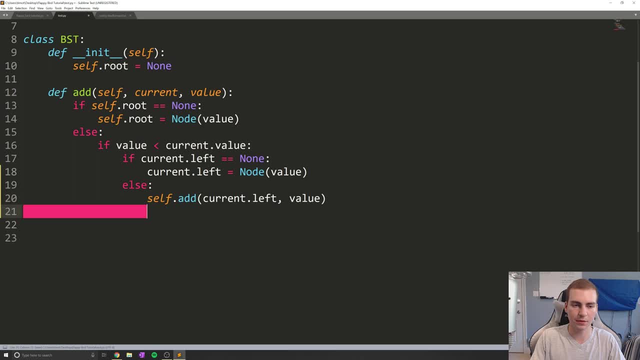 value. I'm going to discuss what this does in a second, But let's move on to the next one here, Alright, so if we've compared our value and it's not less than the current value, then it must be greater than or the same. So in this case, I'm just gonna do an. 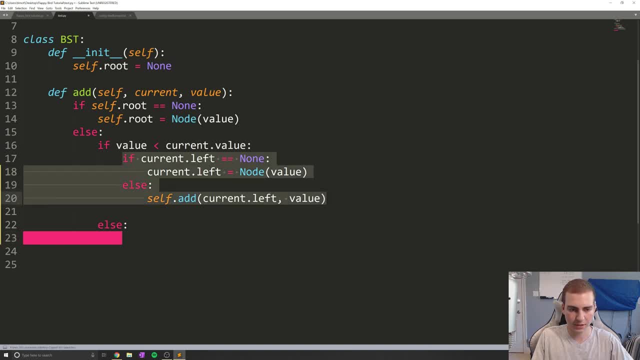 L statement And I'm going to say else and I'm literally just going to copy this, but change this to the right side of my tree. So in this case I'm going to say: if current dot right equals none, then current dot right equals node value. Otherwise, self dot add. 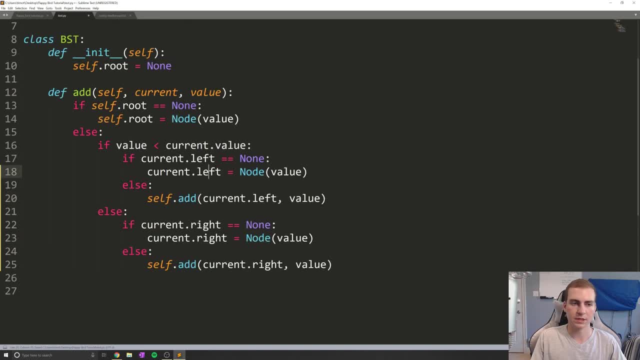 current dot right value. Now let's walk through exactly how this add method works, to make sure that everyone's on the same track here. I'll get my drawing tablet back out so that this is a little bit neater when I'm drawing, Alright, so let's go back into this, Okay. 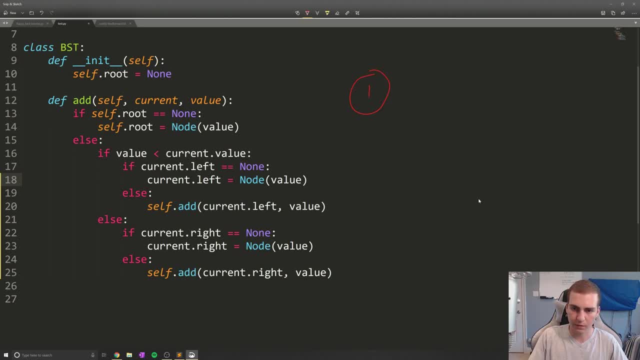 so let's say we have a search tree And it looks something like this: we have one and we have three, or I guess that can't really be three. let's make this a seven, that's a seven, that's a three. And let's say this is a nine, like right here, And I want to add the value two. 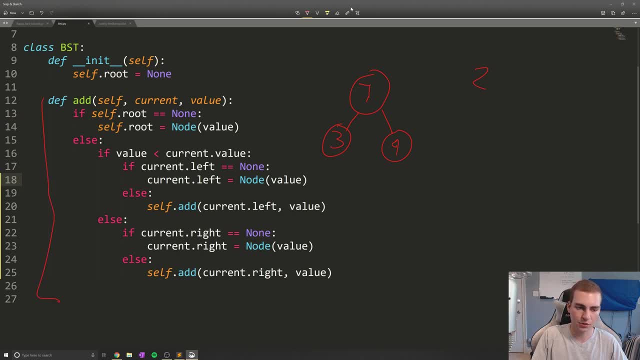 into my search tree. Well, let's go through kind of this method that we just wrote here and figure out what we would do. So we're going to pass. current is going to be the root node to start. So, whatever the root is, which, in this case, is actually just going to be, 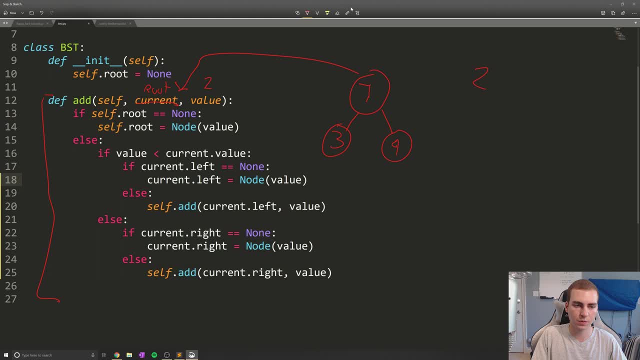 seven, right, And then we're going to pass the value two. So we're gonna do is we're gonna say: if self dot root equals equals. none does it know it doesn't, So we'll move on to the next L statement. here I'm going to say: if value is less than current dot value. 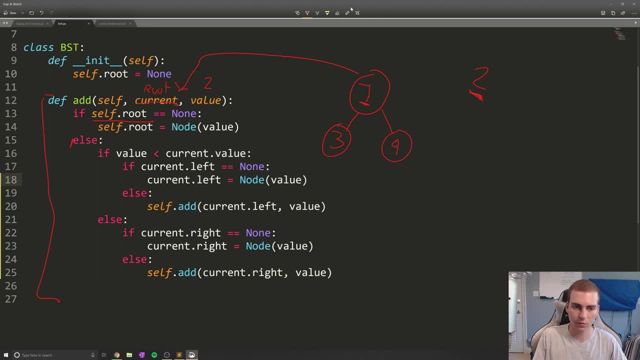 So, if this value two is less than this value seven, which it is, we're going to say, if current dot left equals none does it know it doesn't- then what we're going to do is call this method again, with now the new, current node being current dot left and the value 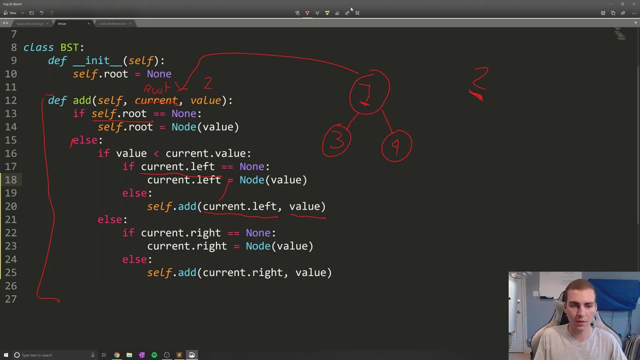 being again two. So we're going to come up here and call this again, But now, if I can get my racer out and just erase some of this stuff, this is no longer going to be root. this is actually going to be the left node of root, which is going to be three. So now the current node. 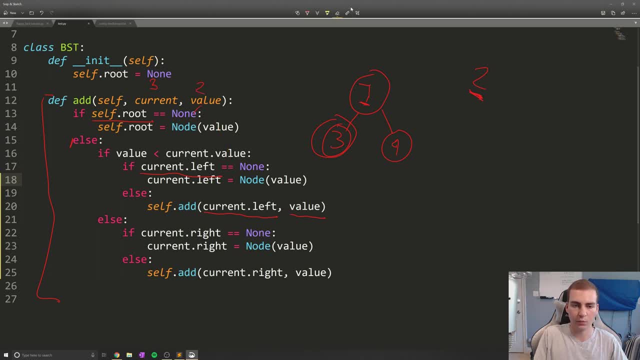 we're looking at is three. the value is still two. And we run this method, the exact same one more time. we check, you know: is the root equal to none? Obviously no, it's not. Then we come here to the L statement. we say: if the value is less than current value was. 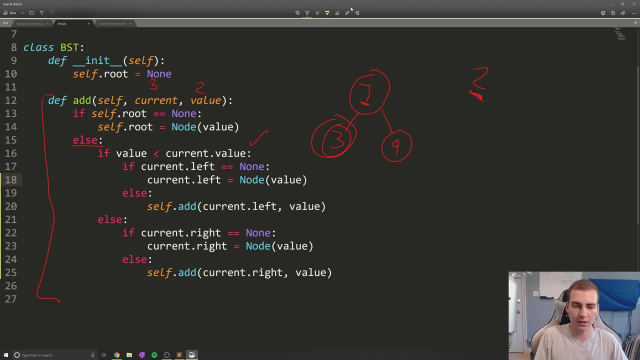 two less than current value. Yes, it is. So we go into here. we say if current dot left equals none, is it? The left of three is none. So what we do is we now add in our new node, which is two. 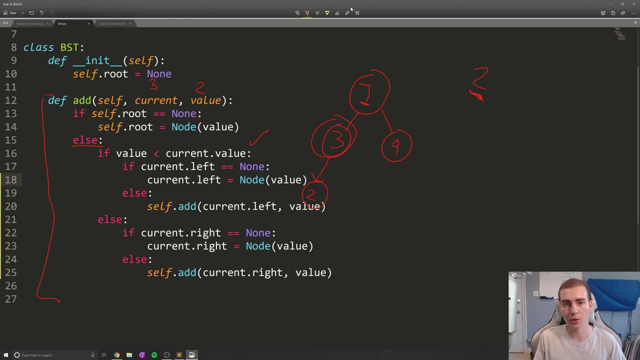 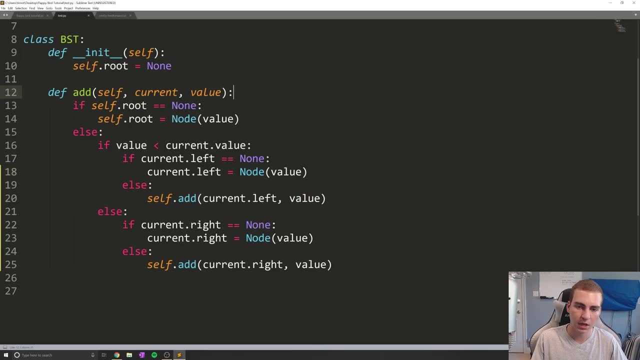 And that goes in the correct place, And we could do this for any example, any number, And this will work properly, just because of the way that I've written that. So I hope that makes sense in terms of that implementation to you guys. fairly straightforward, Alright. 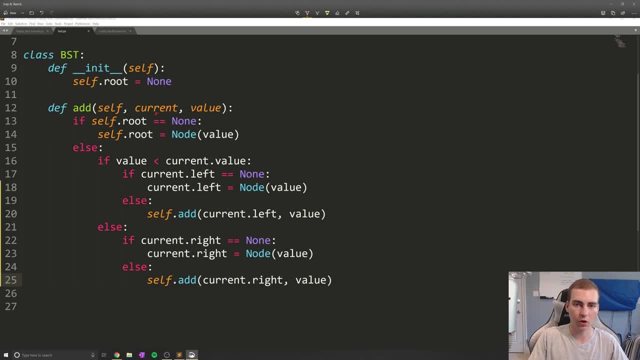 so I want to quickly discuss here how long this method will always take to run. So essentially like: what is the time complexity of adding a new node into our binary search tree? Well, I'm hoping you guys can probably come up with this on your own, but it actually runs in. 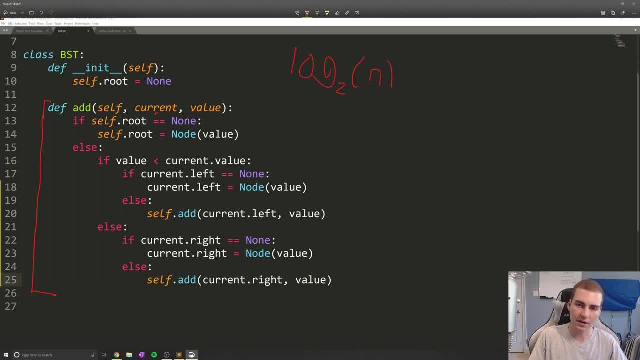 what we call log base two of n time. Now that means that this runs very, very quickly And kind of the bigger that are- I guess binary search tree is, the fastest actually ends up running in in terms of like how much better the speed is getting. So if I just 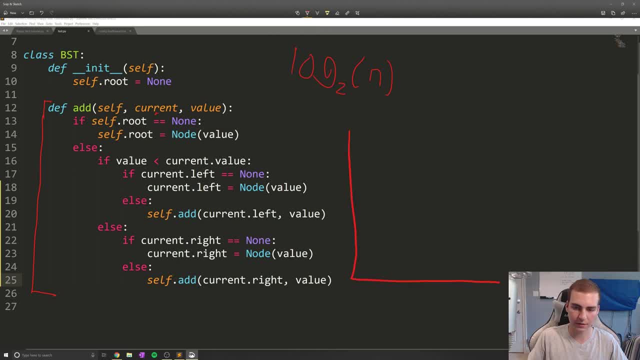 draw. I'm just gonna make this a bit thicker here, But draw a little graph down here. I'll just draw what the log function looks like And you can actually see at least the positive side. it looks something like this. So, essentially, 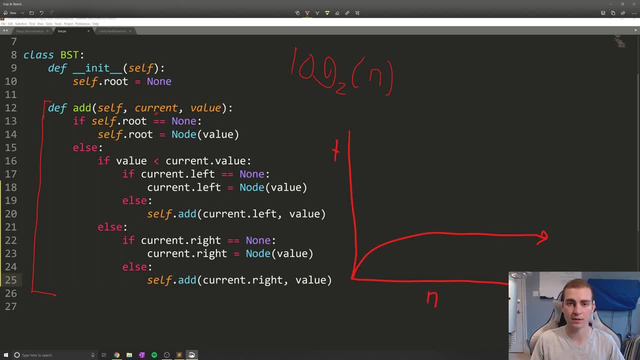 if this is time. so this axis here and this is n, which means how many things we have in our binary search tree as an increases time very slowly increases, which means that this works really well for massive amounts of information, Because as and gets larger, 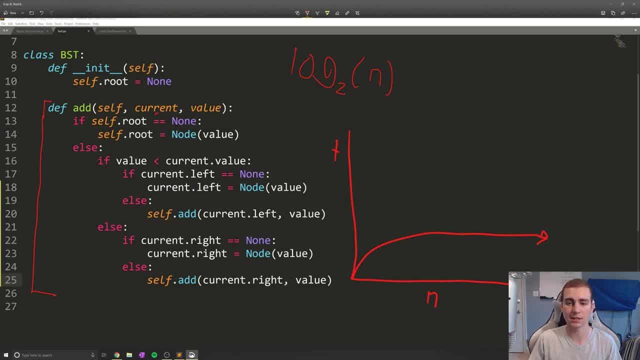 and larger and larger time actually stays fairly consistent and stays pretty similar, And that's why we end up using these types of data structures: Because it's so fast to add elements in as well as to look for elements, which is what we're going to do next. But the reason this runs in log base two of n time and I'm just 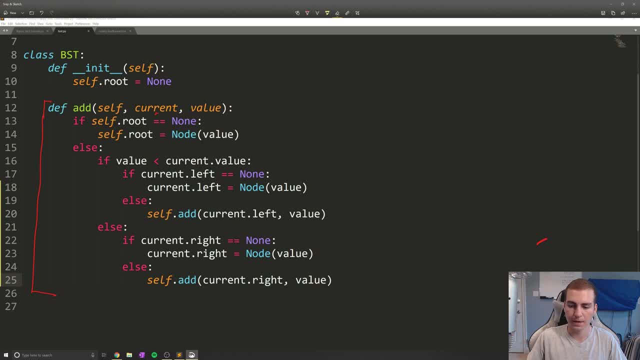 going to erase some of this so that I can show you is because of the way that we store things in the binary search tree. So let's just write a very low show, a very basic search tree here. Let's say: this is seven, this could be- I don't know- three, this will be four. 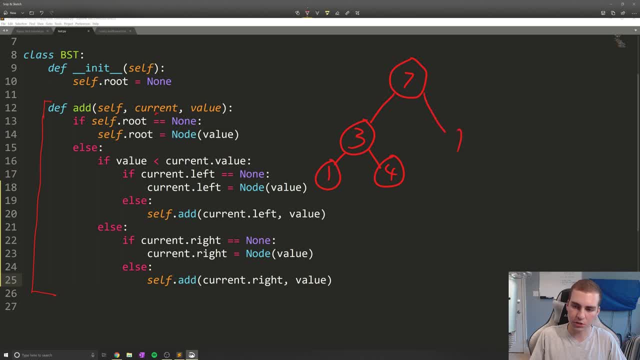 we'll have a one here. I just need to have a few branches that we can actually do a decent example. say, this is 11. And this is eight- Okay, sweet. So this is our binary search tree. Now let's say I want to add in the 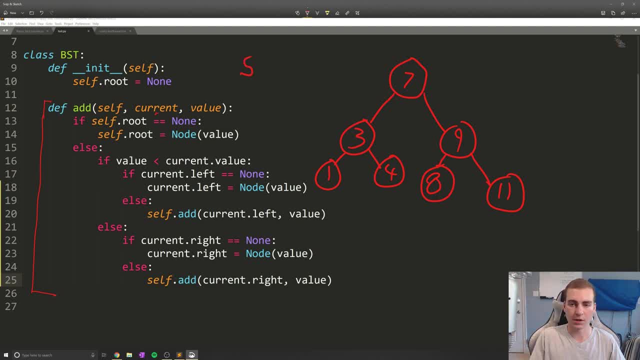 elements five. Well, what's the process of doing this? Well, we first start by comparing five to seven, And when we compare five to seven, we immediately know whether we need to go to the left of seven or to the right of seven, And in this case, we need to go. 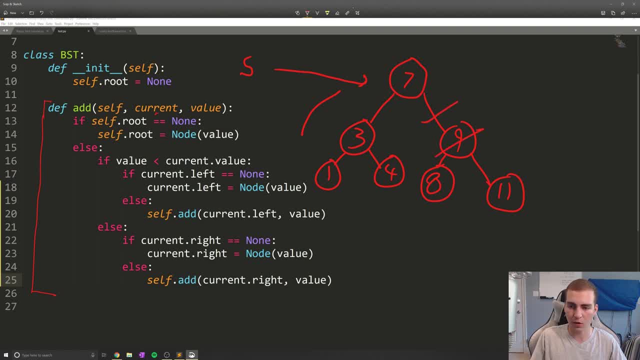 to the left. So what we actually end up doing is eliminating all of these nodes. here we from possible what we possibly have to search through on the binary search tree. So we've essentially cut the tree in half And we've also eliminated seven, actually, because we 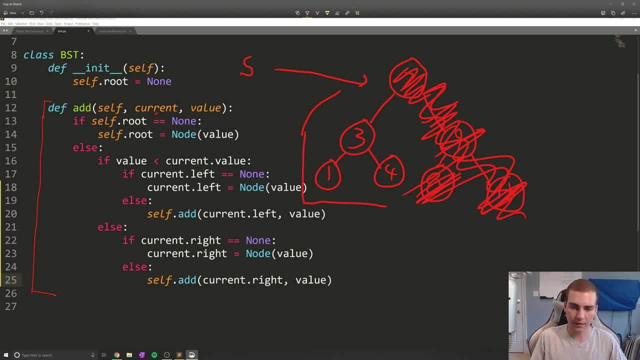 no longer need to look at that Now. what we're doing is we just have this smaller tree that we need to look at. So we now compare five to three and we see: is five less than three or greater than three? well, it's greater. So what we actually end up doing is cutting. 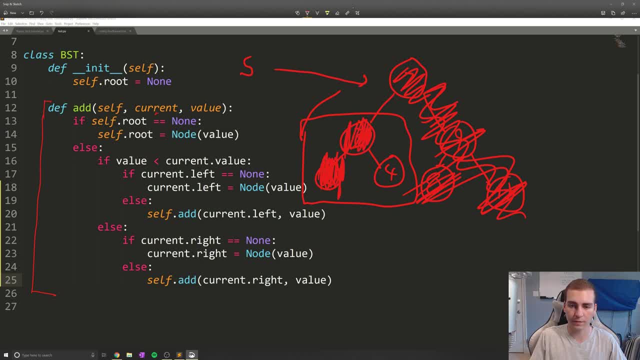 off this entire left branch here of one, and even cutting off three as well. And now again, we've cut this binary search tree in half. So the smaller one that we were just looking at, we've cut it in half And now we're left. 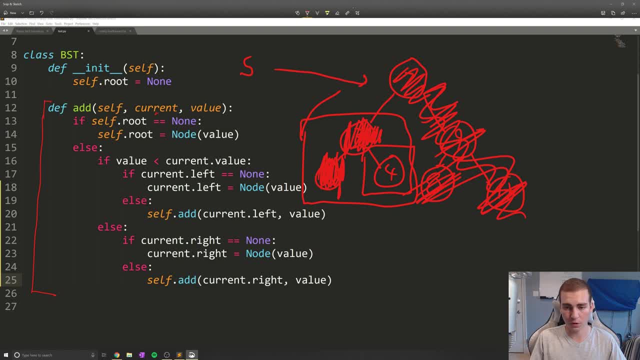 with just this box here- I know this is messy- of four And what we do is we either go to the right or the left And there we go, And then we cut off four And we're done. we've done that in pretty much three different operations. Now, as the tree gets larger and larger and 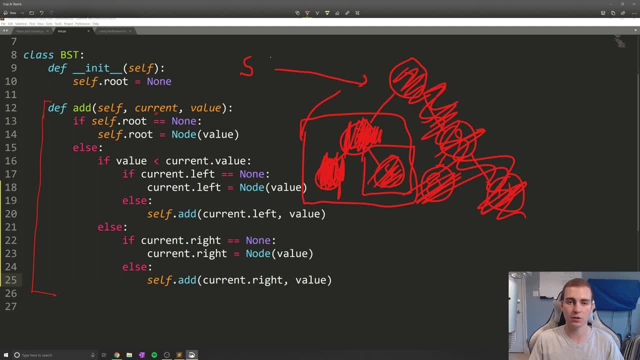 larger, we still don't have to do that many operations because we keep cutting the tree in half and in half and in half and in half until we get to where we need to go And that's why that runs so quickly And that's why it's log base two event. I hope you guys kind of understand. 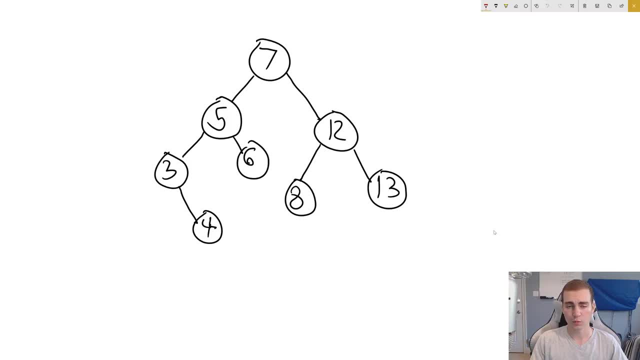 that I'm not going to go into much more detail about that. Alright, so traversing a binary tree. Now, there's three main ways to do this, And the first way we're going to talk about is what's called pre order traversal, Now that you also have post order and in order. 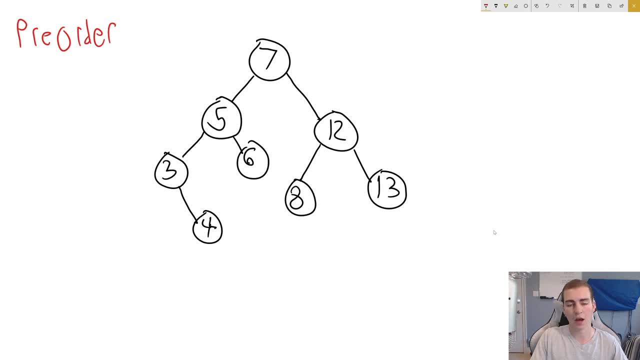 but pre order is kind of the most intuitive, I usually think, and these are pretty straightforward. Now, the first thing to talk about here is we have some kind of idea of visiting a node. So typically when we traverse or look through a binary search tree, we're trying to do something. 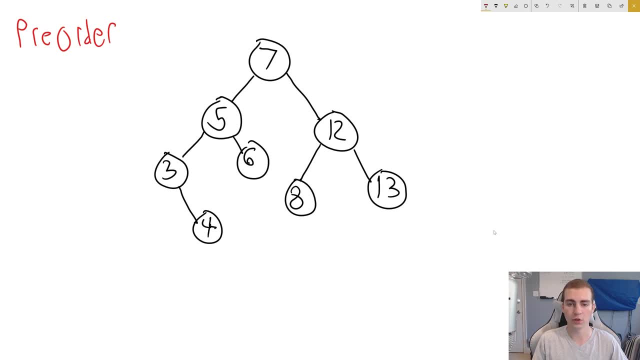 we're either trying to find a specific node or we're trying to, you know, print out all the nodes or collect all the nodes. we're doing something with them. Now, when we actually do whatever operation we want, maybe we're checking something or adding something to. 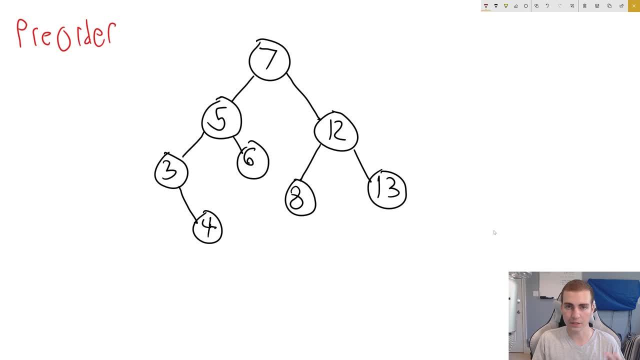 a list. we call that visiting. So when we actually visit, the node is very important because that is kind of how this traversal works. Now, the first order, which is called pre order, simply means- and I saw righty here, actually, what am I doing? visit, go. 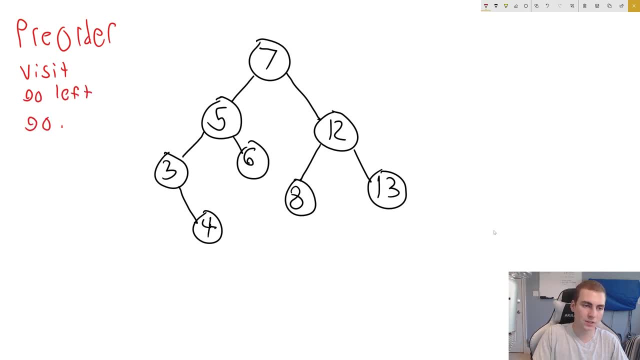 left And then go right. This is what this stands for. Now, it's pretty straightforward. Essentially, what we do is, when we're looping through the tree, we start by visiting the root node, which is this one, so we visit it. Now, when I visit a node, I'm just going 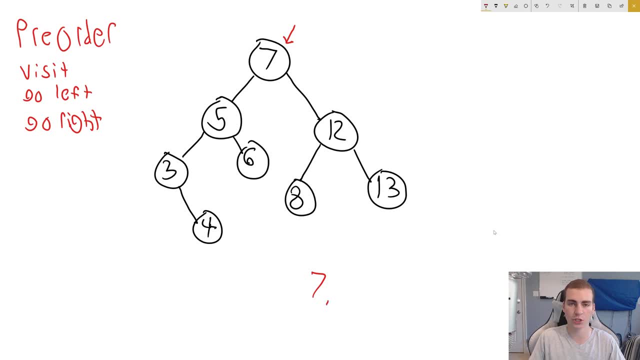 to write it on the bottom of my screen So you can see the order in which I'm doing things. So seven is the first node we visit. maybe we're doing something like this. let's say, we're doing something like this, let's say, a tree. So now we're gonna do something like 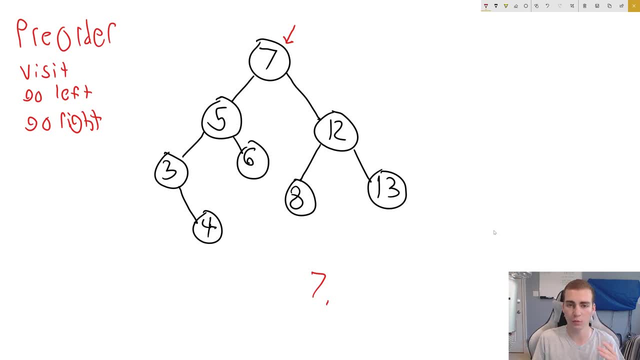 this, And then we're gonna do something like this. let's say we're doing something like this, we're looking for a node, we check it doesn't know. we're looking for. whatever it's doing, we visit it. Now, what do we do? we go left. Alright, so let's go left. So we do now is: 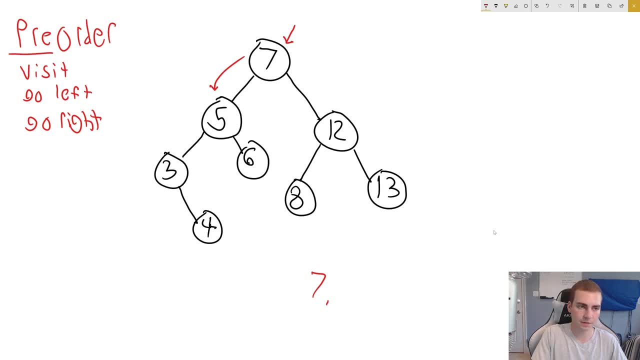 we go left and we go to five And we repeat this process of this pre ordered traversal on this node. five now. So even though it says go right as the next step for seven, we need to first do five because we've just gone to the left. So what we do now is we visit five. 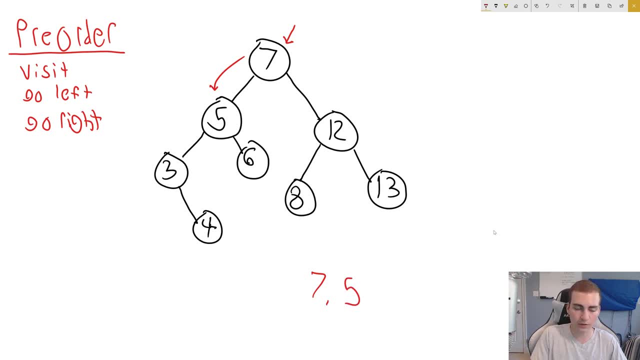 which means I write it down here. And then, what do we do? we go left. So we move left again And we visit three, which means I write three down here, as if we've been to three already. Now what do we do? We go left. Well, when I go left here, there's nothing here. 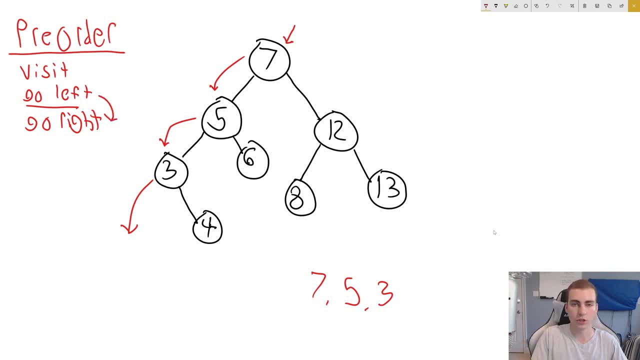 So what I do is I move on to the next step, which is: go right. So now I go right and I go to four. Okay, so now we visited four, Alright, so now that we've done that, what do we need to do? we need to do that, So we're going to go left and we go to three, And 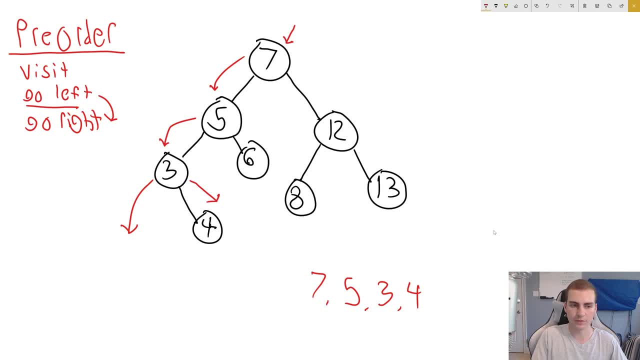 we visit five, And now we're going to go right And now we're going to go left And we visited four. Now that we've done that, we still need to kind of go back up the ladder and go right, because we've just finished going left. So, essentially, from seven we went left to five. 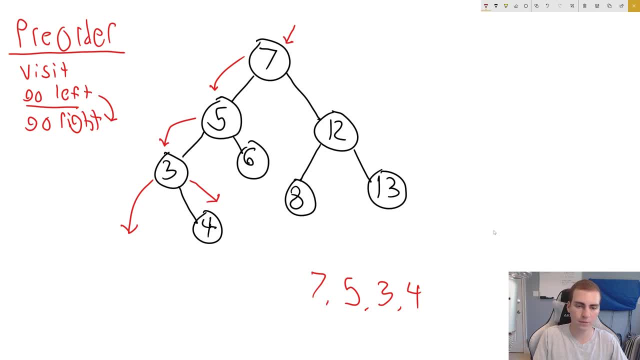 we visited five. we went left from five to three. we couldn't go left from three, so we went right, And now we've completely gone as far left as we can go. So we start coming back up And we go: Okay, we go to five. Well, we went as far left from five as we can go. 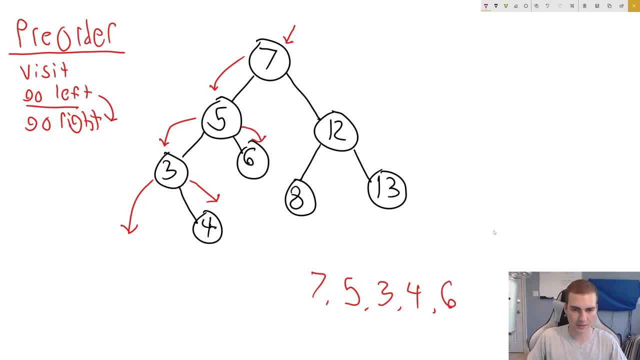 So now we go right and we visit six. And now, well, we've go back up to seven. we've to seven, because we've gone as far left as we can go. And what do we do? we now go right. 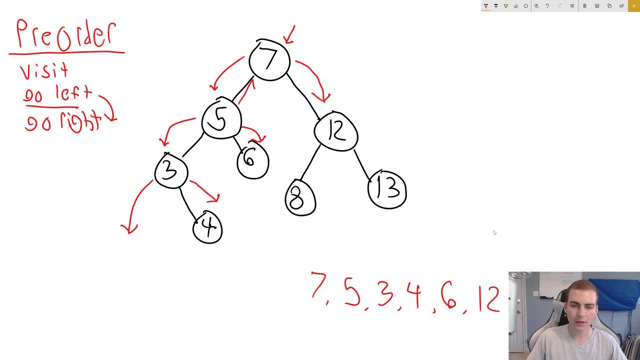 and we go to 12.. So now we visit 12. And from 12, we follow this process: we visit, we go left and then we go right. So we visit it And now we go left to eight, which is here. 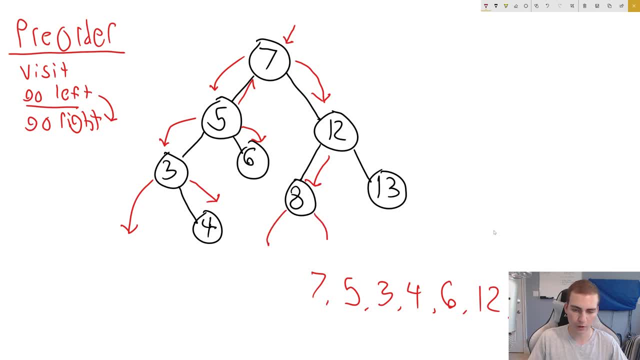 And we've followed this process. So we visit it. we go left, we go right and we can't do anything there. So we come back up to 12.. And now we say: Okay, we've gone as far left as we can go. we couldn't go right. So now we go right over here to 13.. And we follow. 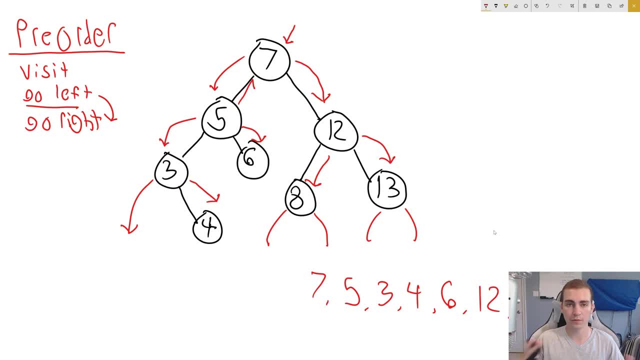 this process we go left and we go right And once we've reached a point where we've pretty much completed this process, we are done And we have traverse the entire tree And that is what we call the pre order traversal. So, visit, go left and go right. So once you, 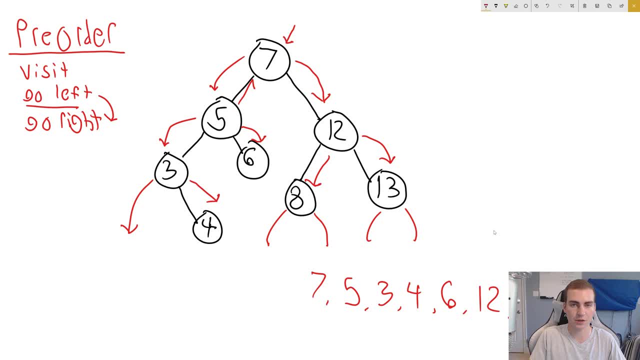 end up going left, then you know you follow the same process on that left node And continue and continue and continue until you can't go left anymore, 12. And then you start slowly going right and moving your way back up the tree. If you simply 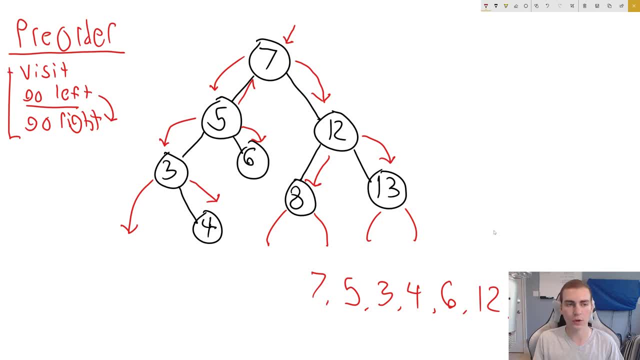 follow this process: visit, go left, go right. you know to do pre order And that is how that works. Now give me a second to clear the screen. I'll be back with in order, Alright, so what is in order traversal? Now? it's a similar to pre order, just a little bit different. 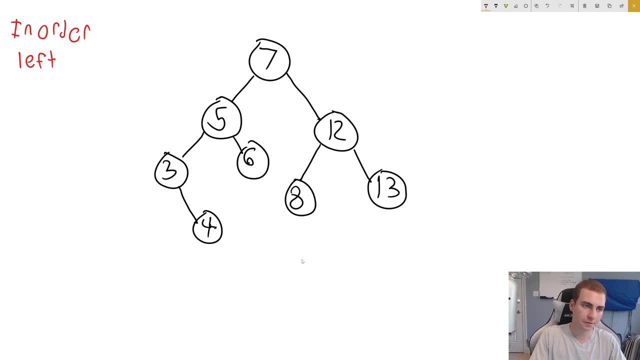 What we do is we go left visit And then we go right. That is the in order traversal, and you guys are gonna see why we might do something like this as I start to write down the nodes that we're visiting. So we always start at the root node. Now we're starting. 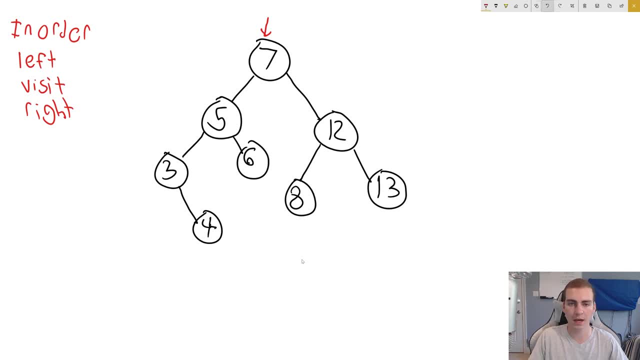 at seven. But notice that I'm not going to write seven here yet, because I haven't visited seven yet. So when I visit it, that's when I write it down. I haven't visited it. So the first thing I do when I get to seven is I go left. So go left here to five. Now when 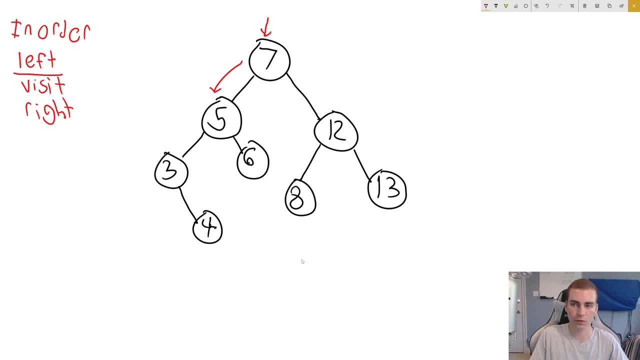 I go to five. what's the first thing I do? Well, I do the first step here in the in order traversal, which means I go left. When I get to three, what's the first thing I do? I go left. Now I can't go left from three, So what's the next thing I do? I visit it. So 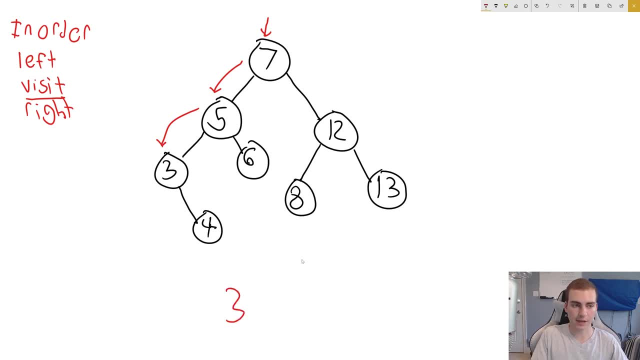 I write three down here. Now what's the next process after visiting? Well, it's going to the right. So what do I do? I go to the right Now from here. I follow the process left, visit right. left can't do it, Visit Right, Can't do it. Come back up. Okay, so let me just. 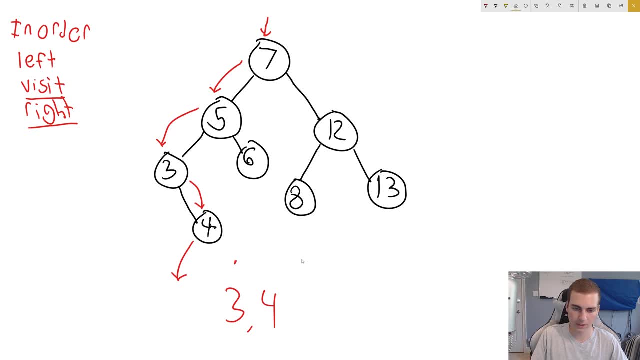 get rid of these arrows here, Just because I don't want to have them. Alright, so they there, we go, So we go to four, then we come back up. Now we've already visited three, So we go to five. And what's the process? visit five because we had already gone, left from. 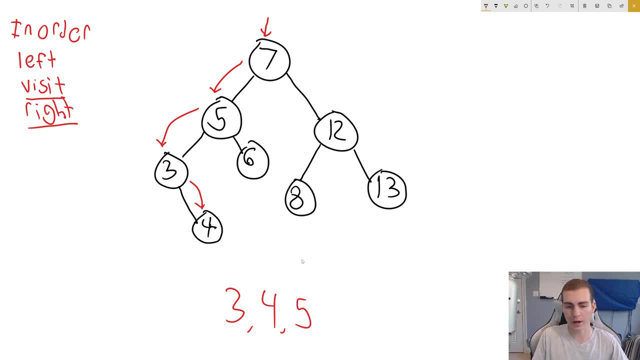 five, right. So now we visit five. And now, what do we do? we go right. So we go to six, now, which is here. And what do we do? we left visit, right. Well, we can't go left, we can't. 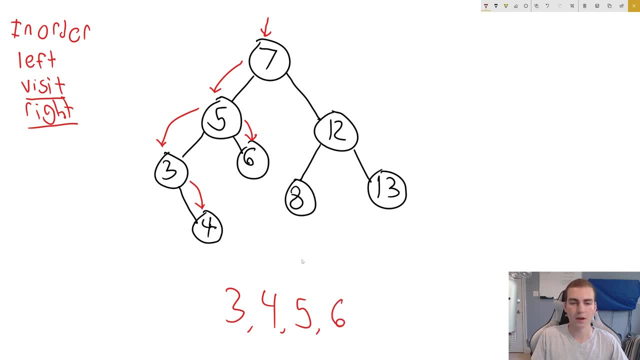 go right And we visited in between there. So now we have six, And now we come back up to five. We've gone right from it. Five is done, We're at seven. Now what do we do? we visit seven, Because you know we already went left. Now we're back here, So we visit. And now what? 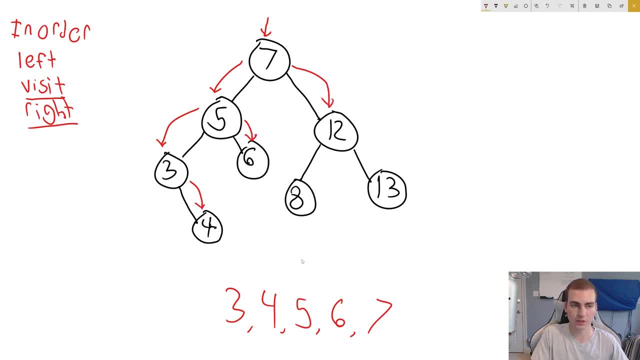 do we do? We go right. And what do we do from 12?? Well, we start, we go left, So we go left. here, this guy goes left, visit right. so we visit him eight. then we come back up to 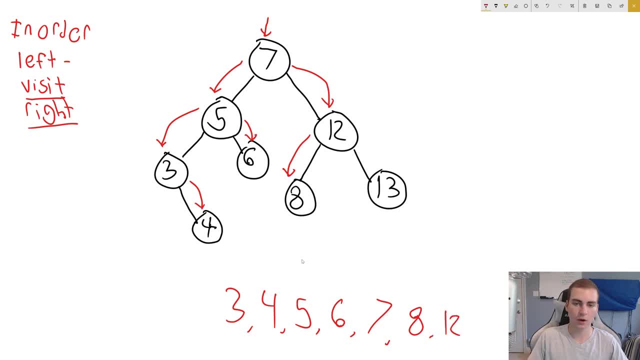 12. We visit because we've reached 12. Again, And now we come over to 13. We go right, we visit 13.. And there we go. That is the in order traversal, And notice: this gives our numbers in order. So left visit right. 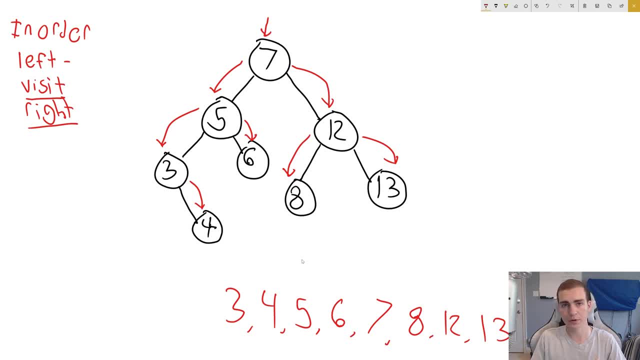 Now, if you wanted to go from greatest- like the largest number- to the smallest number, you could do right, visit left, And that would give you the opposite order, because you would go as far right as you could, And then you work your way back, going left, and you would 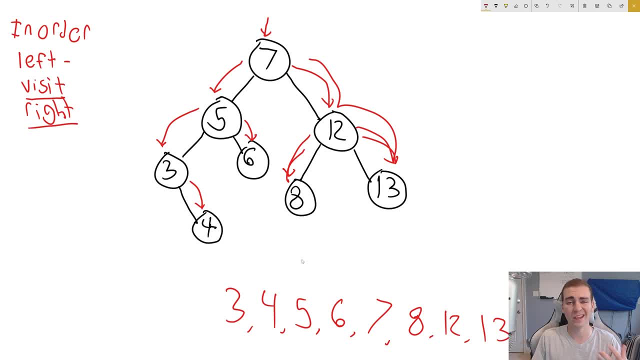 get this kind of flipped, So you'd have 13 at the start and three at the end. Anyways, that is how the in order traversal works. going to clear my screen and I will be back with post order. Alright, the post order traversal is kind of the opposite of pre order, So I'm 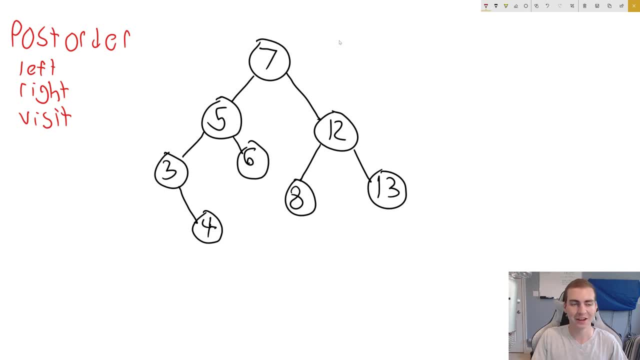 pre order: we have the in order traversal. we have the in order traversal. we have the left right visit, or sorry, we have visit left right and post order: we have left right visit. So what we do here is follow the same process that we've done before. 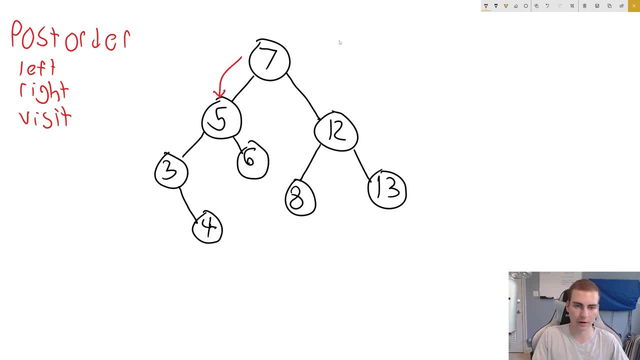 except we go left right visit, So we go left. Alright, we're here at five, Now what are we doing to go to left? we go left. Now what do we do when we get to three? Well, we can't. 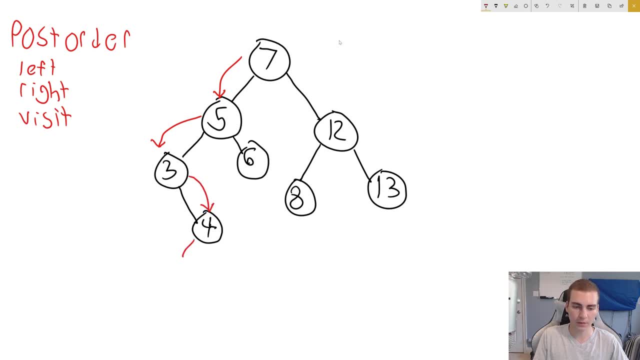 go left. So what do we do? we go right Now from here. we go left, right visit. so we write for because we can't do anything from there. So we visit for as the last step we do we do. we come back up to three here And now what do we do? we visit three because we 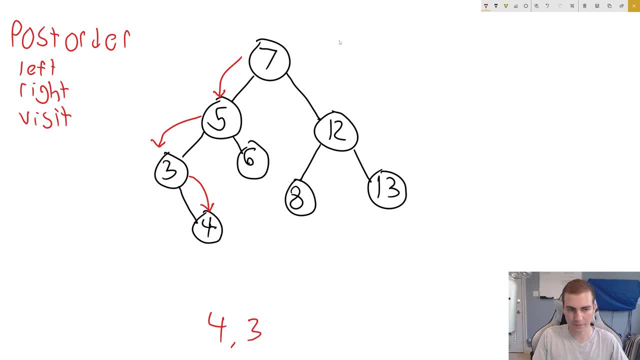 had gone right. So we write three here. Now we come back up to five. we go right, because that's how we had just gone left to go to three. So now we go right to go to six. we go left right, visit. So we write six here. Now we come back up to five. we can finally. 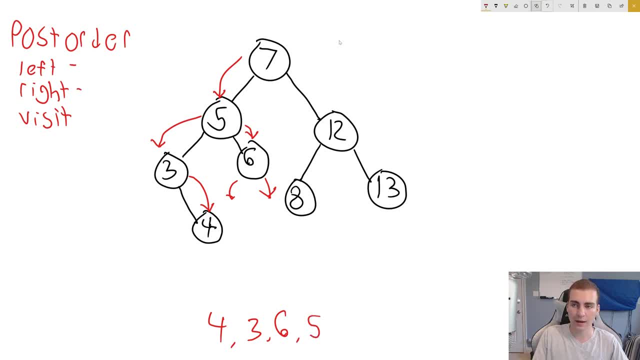 visit five because we had just gone left right. Now what do we do? we come back up to seven and we go to the right. So now we go 12.. What's the process here? left right visit. So we go left here to eight. Obviously, from eight we can't go left or right, So we need to visit. 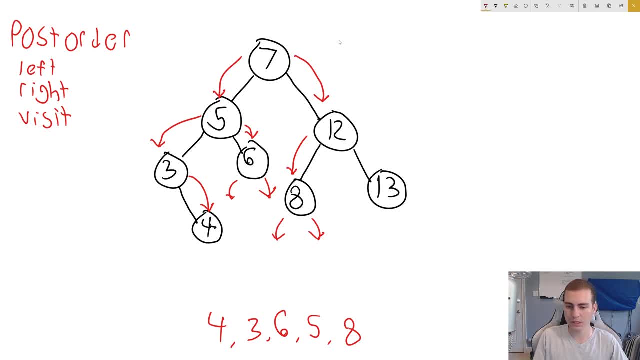 which we do. then we come back up to 12.. What do we do? we don't visit, yet we go right, because we just gone left, So now we're going right, So we go 13. Obviously, we can't go anywhere. 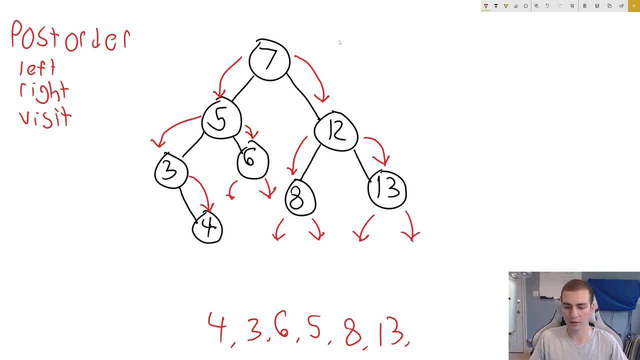 from here, So we just visit it. Now we come back up, we can finally write 12, because we just went left, right And now finally back up to seven And we go to the right. So now we go to 12.. What do we do? we come back up to 12.. And now 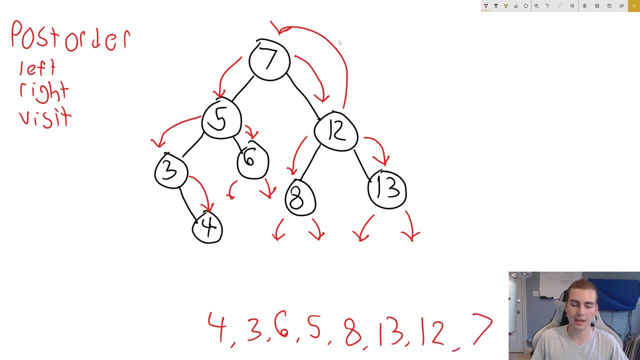 we come back up to 12. And because we had gone left right from seven, we can write seven at the end, And that is our post order traversal. Notice that you're always going to get your root node at the very end of your post order traversal And that is just the. 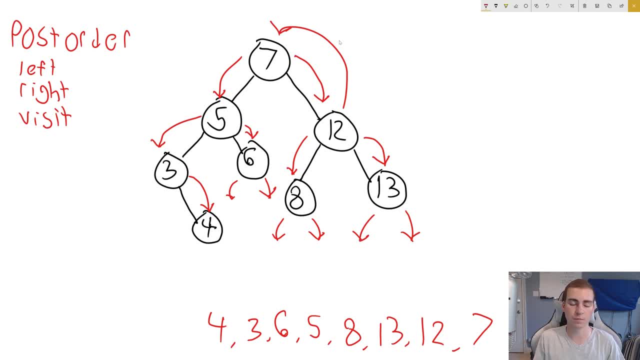 way that it works, Because left right visit And since this was the first node, to repeat that process, not until everything else is visited are we going to visit that root node. There's different uses for all of these. I'm not going to talk about kind of what those 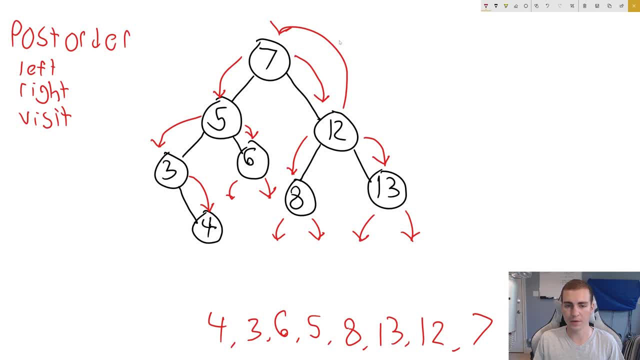 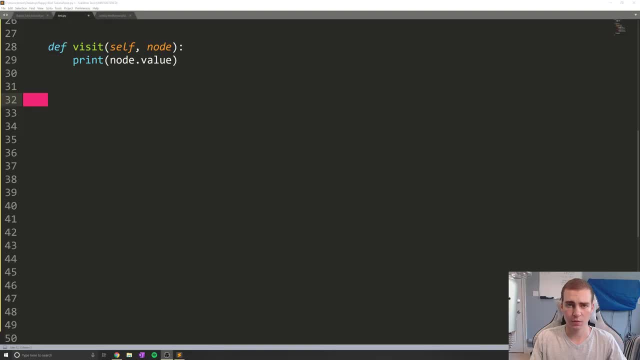 are. you can figure them out as you go, But now I'm just going to quickly show you an implementation in actual code For this, and then we're going to wrap up the video, and hopefully you've learned a bit about binary search trees, Alright, so what I'm going to do here is just quickly program. 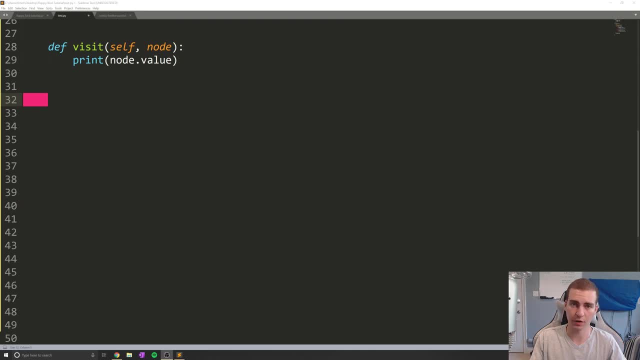 the post order in order and pre order traversal. they're really straightforward. you're going to see how easy they actually are. And just notice, I've created a visit function here which is going to stand for what happens when we visit the node, And in this case, I'm just 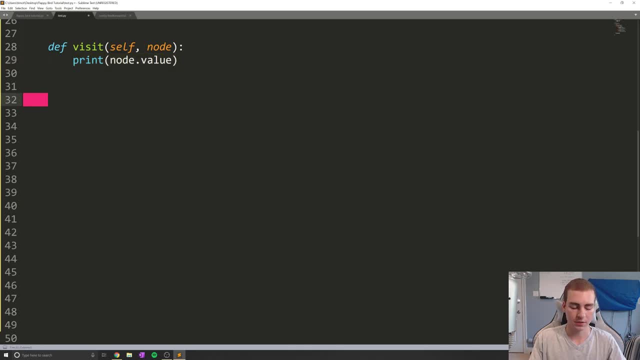 going to print whatever the value of that node is. Alright. so what I'm gonna do here is start by doing pre order. So we're going to say pre order as the name of our method here. it's going to take self And it's going to take, I guess, current as the node that we need there. Alright, so what? 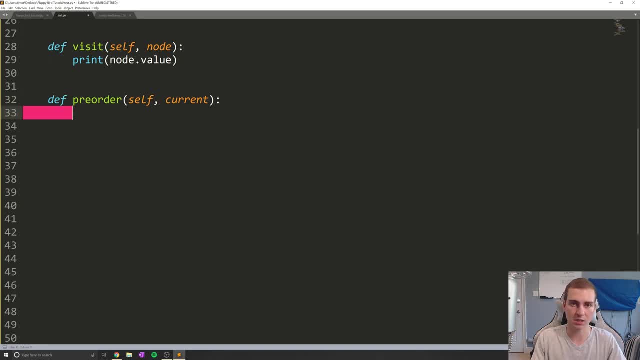 we're going to do inside of pre order is simply follow the process of visit left right. So what we're gonna do is we're gonna say visit, in this case current, so I'll say self dot visits, this is proper. And then we're going to go to the left and we're going to go to 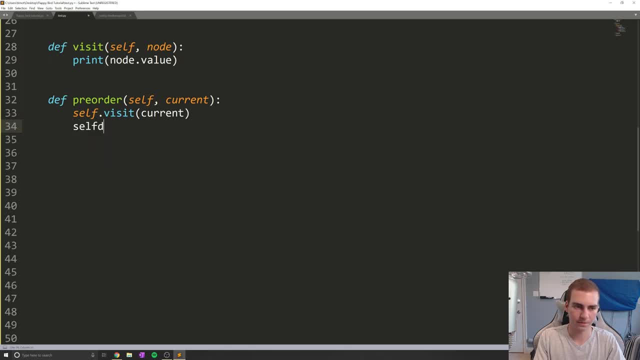 the right. So to do that? we're going to say self dot pre order, Like that, And then we're going to go current dot left, like that, and self dot pre order And, in this case, current dot right Now. this is all we need to do for pre order. And why does this work? Well, 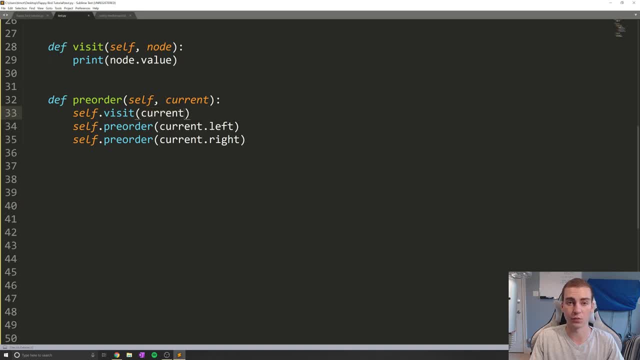 exactly what we've shown before. So current is going to always start off as the root node. So we're gonna do is we're gonna say self dot visit. we're going to visit this root node. So print that out, because that's what visit does here. then we're going to go to. 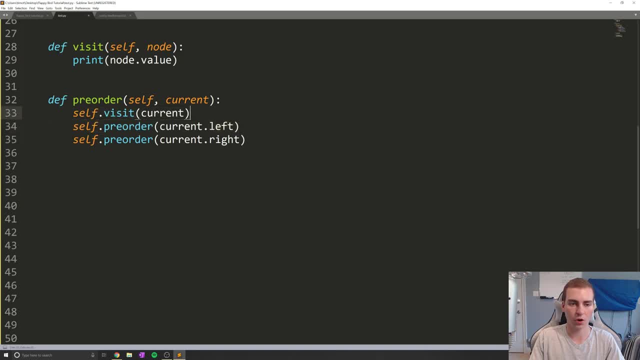 the left of the root node And call this pre order function on the left of the root node, which is now going to pass. whatever that left node is, we're going to visit it, and then we're going to go to the left and we're going to go to the right, And this is recursively going to call itself. 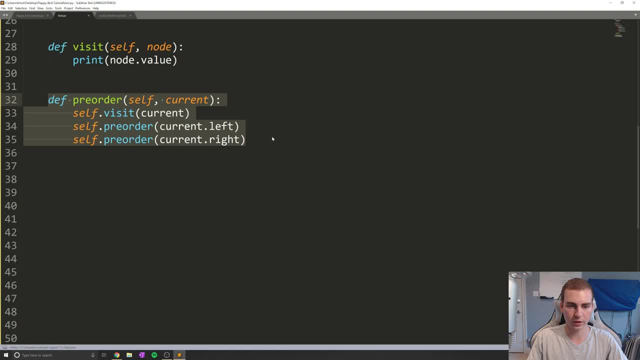 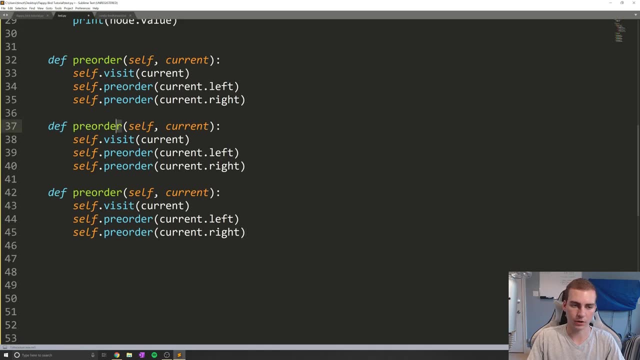 and do the pre order. Now. I'm just going to copy this and really quickly show you post order and in order. But it's just a matter of moving around some of the statements in here So they follow the correct order. So I guess we'll do in order here. So in order. 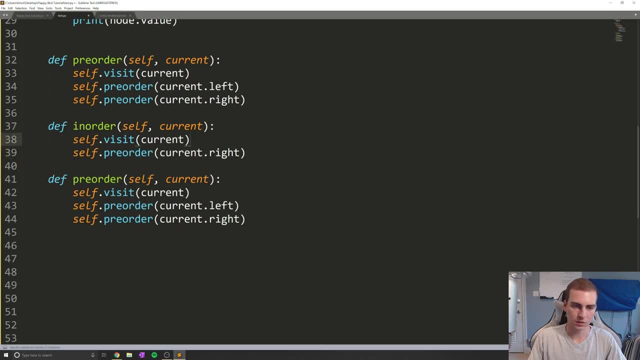 is just going to mean we're going to go left, visit right. Let's move the left up here And that's all that we need to do And post order. we'll simply put the visit at the bottom and change this name to post order, Like that. What am I doing? 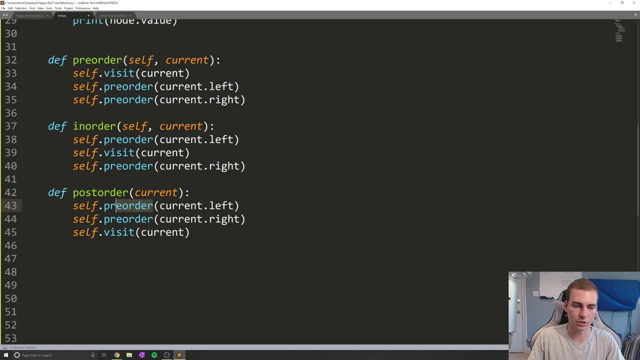 here Like that, And then obviously I mean we need to change these to be post order and in order. But you guys get the point here. That is kind of how that works And that is all that we need to do For the implementation. I'll just change these because it's going. 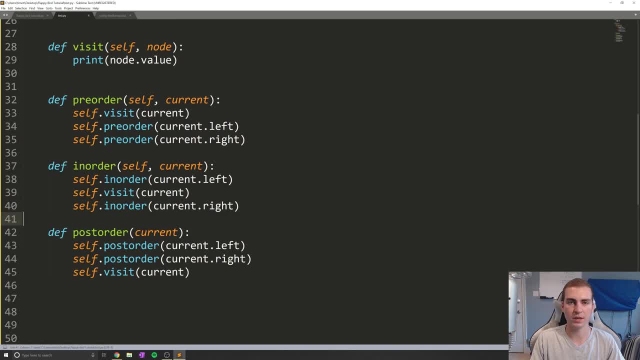 to bug me if I don't, And that is kind of how we can traverse through a binary search tree. Now, there's tons of things you could do with a binary search tree. I literally could have made this video like 10 hours long, of the amount of different problems you can.